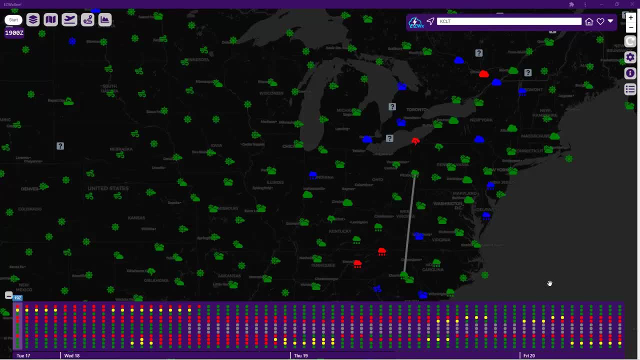 on numerical weather prediction models, how to best use them in the Easy Weather Brief application, And certainly there's a lot to talk about. I want to first of all start out, before I get into the main topic here, talk about one thing that I've gotten a lot of. 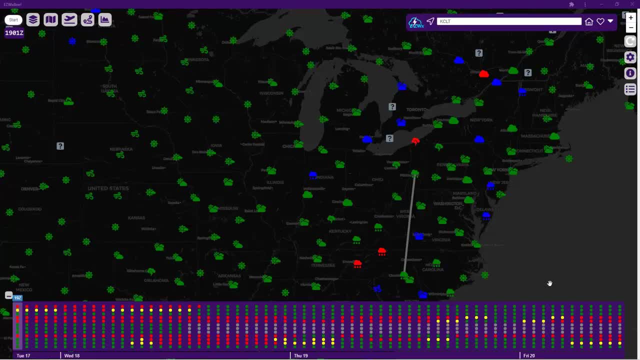 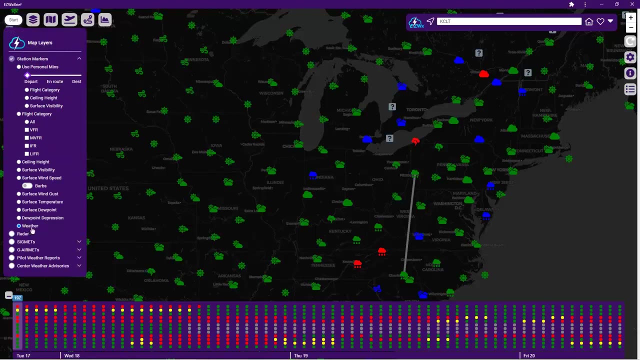 questions about. and that is when I look at the map- bring up the Easy Map here- and I look at the various different icons. I've got the weather icon up here, so if you go to the layers station markers, notice I have weather selected. It's one of my favorites. 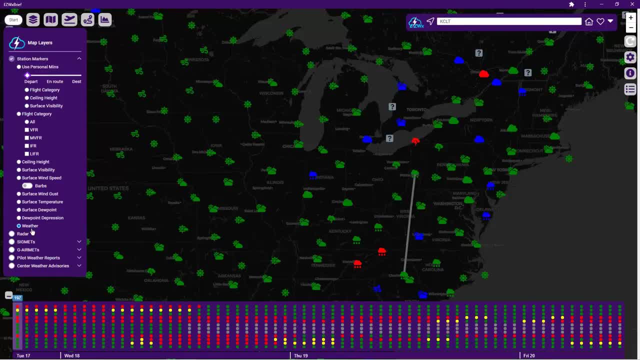 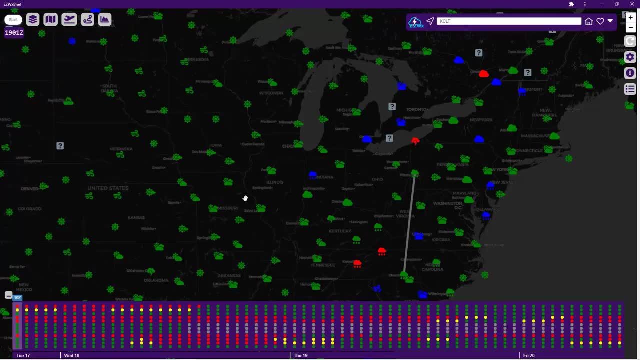 because it provides you with a lot of information with very little trouble to get there and you certainly can understand the impact for ceilings and visibility issues potentially, and just the kind of weather that's occurring. When the map is up and displayed, you'll notice that the departure advisor here when it's 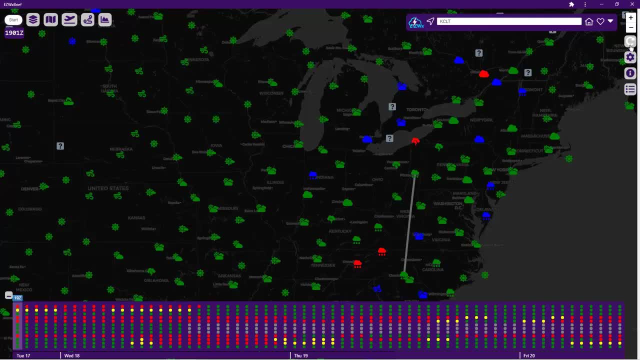 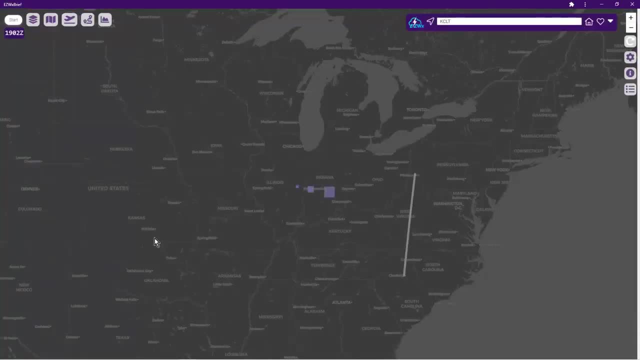 on the very far left side. let me just refresh this to get the latest and greatest information. but you'll notice that on the very far left side essentially it's 1902Z, so the departure advisor will always start at the top of the next hour. So when this comes up, you'll see. 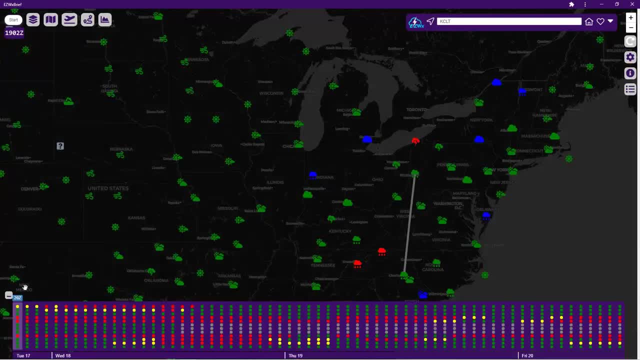 that it will start not at 19Z, but it will start at 20Z. That's because we're looking at basically a forecast for the future, but when the departure advisor is all the way to the far left, that essentially is going to display all the latest observations up. 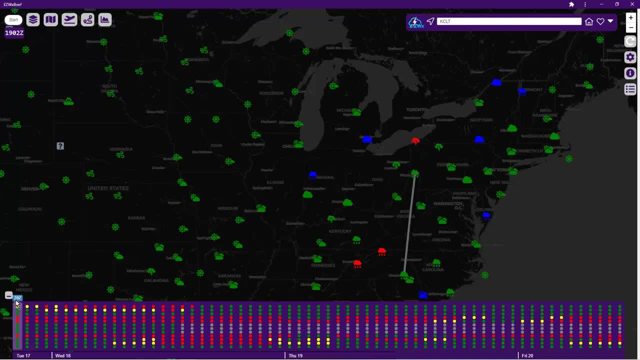 to essentially the current or the latest time, in this case 1902Z, And so if you click on any of the surface observations or airports, the station markers here, you'll notice it does display the information about the surface observation for that airport. 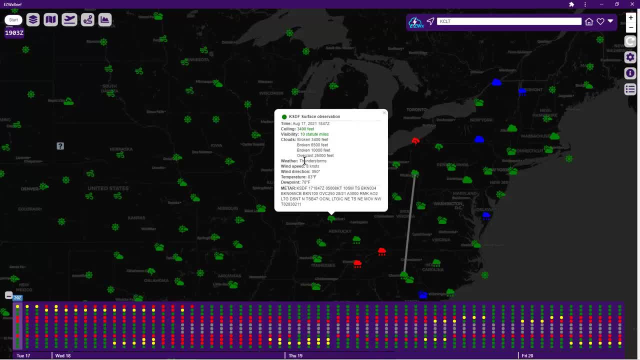 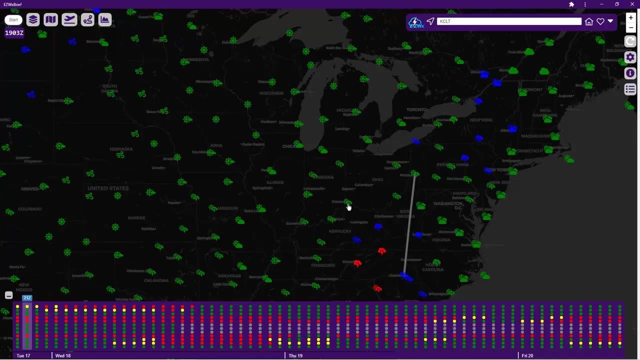 And it breaks it down in a tabular form, so it's pretty easy to understand Once you move the departure advisor to the right by one step. now we're displaying forecasts, Not observations, So this is the easy forecast for Cincinnati and it shows the possibility. 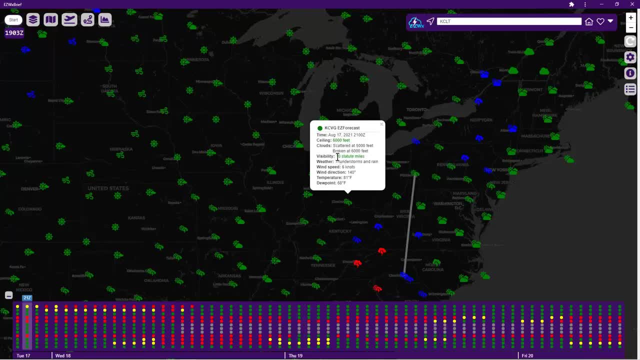 of scattered at 5,000 feet, broken at 6,000, 10 statute miles, thunderstorm and rain, And that's valid at 21Z and that's what's on the departure advisor. So everywhere on this particular map, all of these are valid at 21Z. 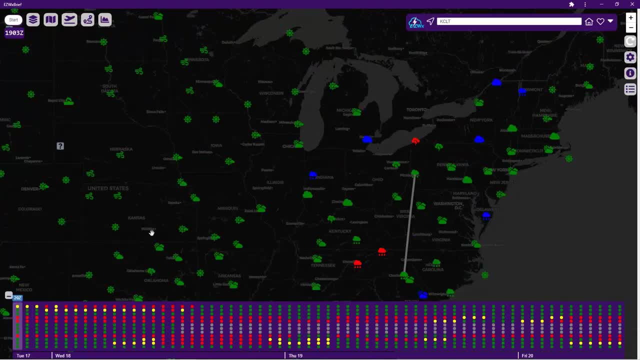 Whereas when you're looking at surface observations, these are valid when the surface observation is taken, So it's 1903Z. this one was taken at 1853Z, so that's pretty pretty recent overall out of Kansas City, And you may even find surface observations. 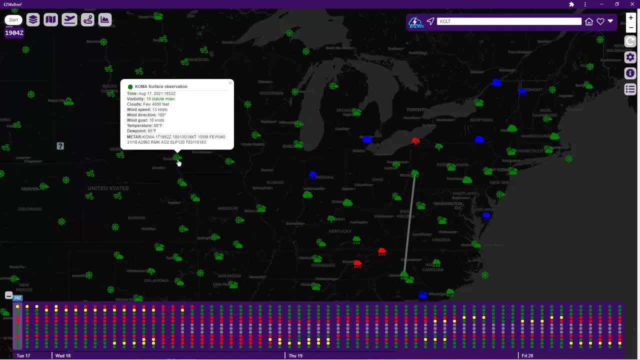 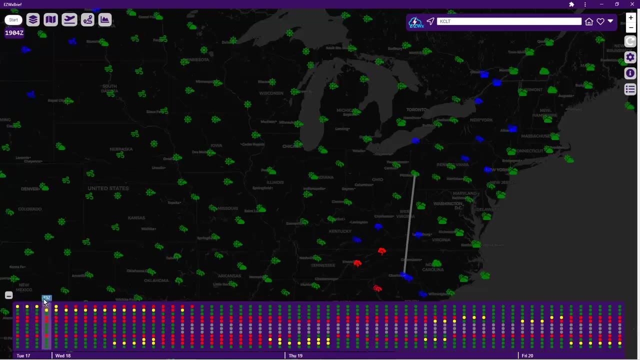 that are much older than that, perhaps even as far back as an hour old. so it tries to show you again the latest observations in Kansas City And here are some of the observations for that particular airport and, like I said, when you move this to the right it: 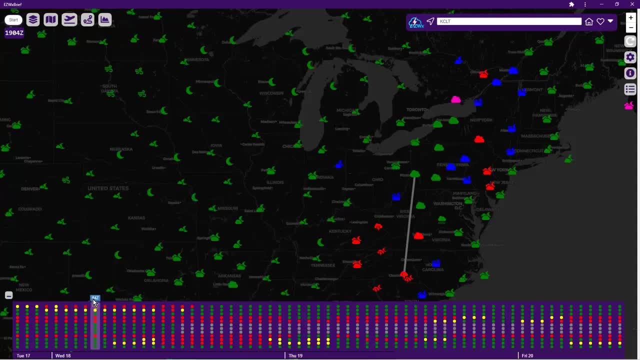 will then display the forecast for that particular time. in this case, I set it to 4z and all of the all of the forecasts here are valid all at 4z at that particular time, and that's independent of whether you have a route defined or 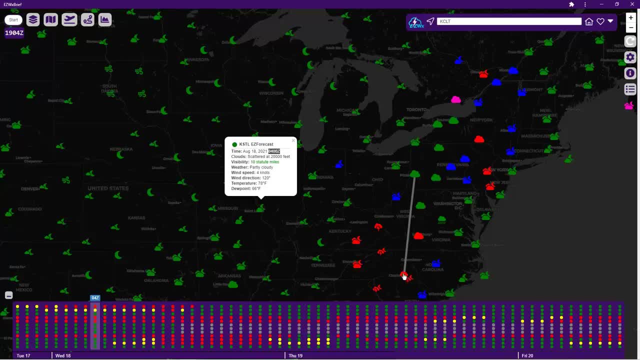 not so. even though the route may take me, let's say, an hour and a half, two hours, three hours, to get to my destination, in that particular case it still only shows you based on the departure time that was set here. so in this case, 4z, 4z. so if 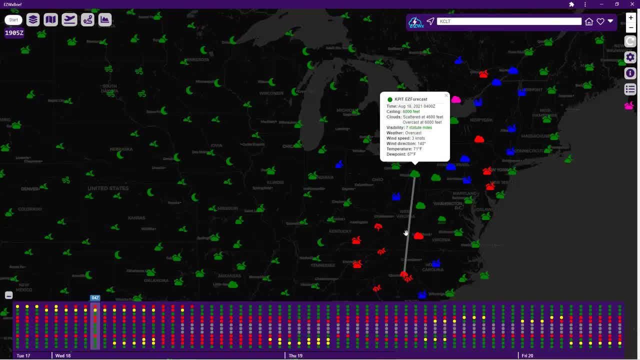 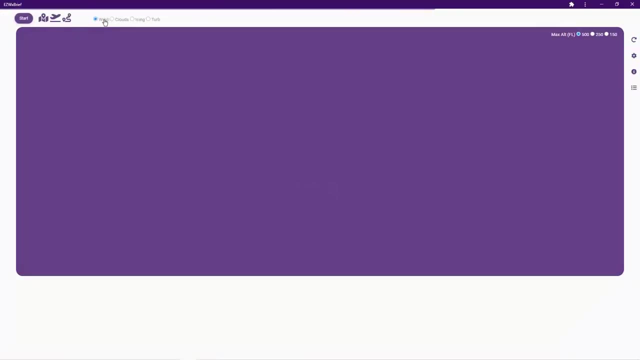 Pittsburgh is my destination airport or my departure airport, doesn't matter. it's always going to show 4z here now when we go to you. the profile view, easy route profile. in that case, it does take into account where you're going to be along the route of flight, so it knows based on the settings. 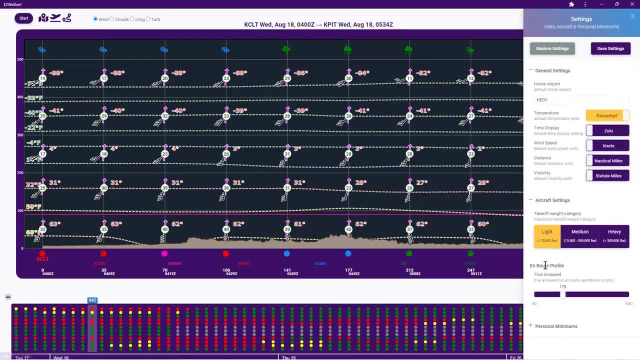 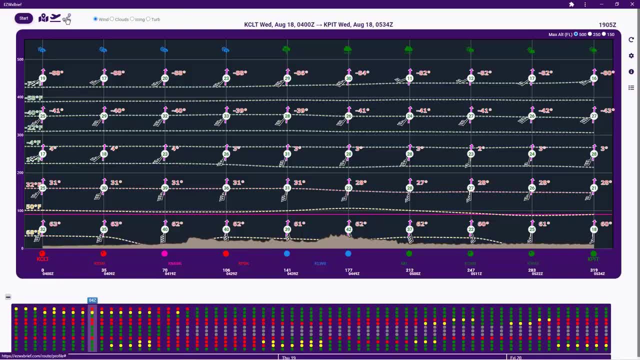 that you have set up here. aircraft settings set up a true airspeed of 179 and in my route I set up and I want to use forecast wind so it's calculated, calculating along the route of flight, how long it's going to take you to get to each of these. 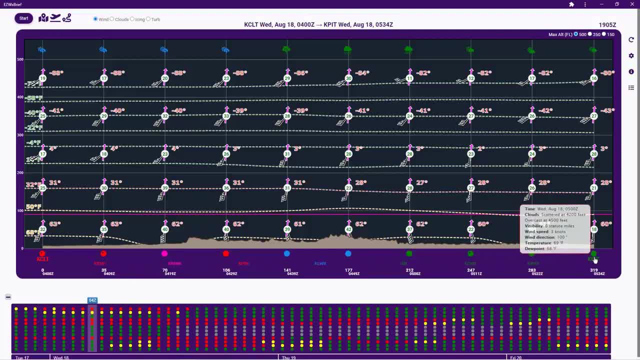 different intermediate points here and eventually to your destination. so it's calculating a ground speed, and so the idea here is that we're at 4z, departing out of 4z, out of charlotte, and so all the data that's at that point is all going to be valid at 4z. 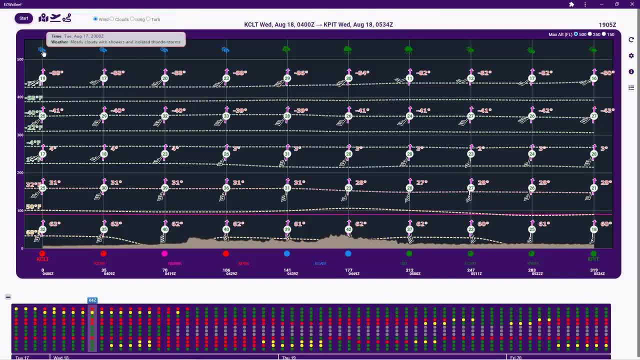 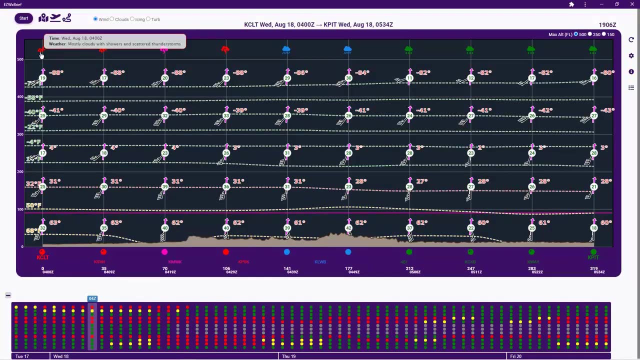 and it doesn't matter what you're looking at. you're going to see the- uh, the case where you're going to be departing at 4z here, and so what you want to do here is: you want to, you want to um, in this particular case, you want to understand that the data is going to be now related to where. 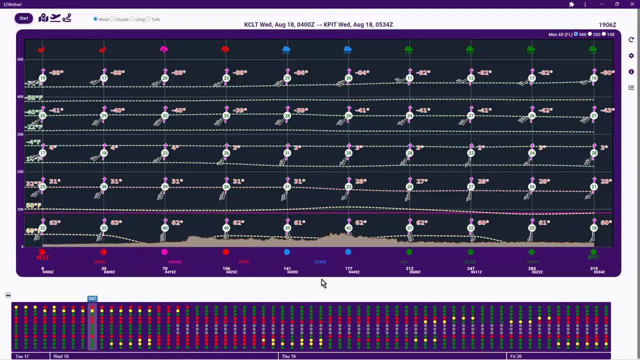 you are along the route of flight, so once we pass over, let's say 5z here- now all the data is valid here, at 5Z, which you see, And so that's going to persist, even though it's 511Z, when you reach this next point. 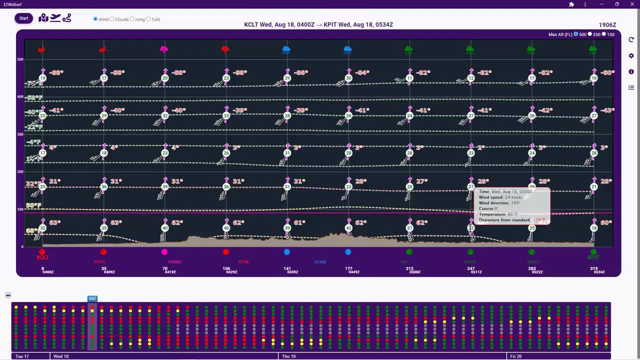 We're still using data from 5Z because that's the latest information. We have hourly forecasts in EasyWeatherBrief, But before 5Z, all these are going to be taken from the 4Z forecast And some of this data, or in this particular case, comes from multiple different forecast models. 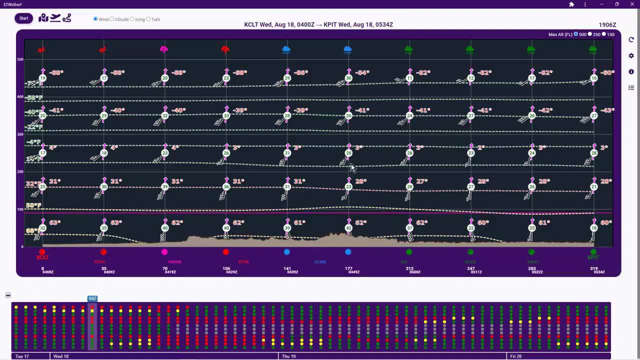 as we'll talk about in just a bit. So the important thing to recognize is that EasyWeatherBrief takes into account where you're going to be along this route and it's going to look at the time from the forecast that they have valid at that particular time. 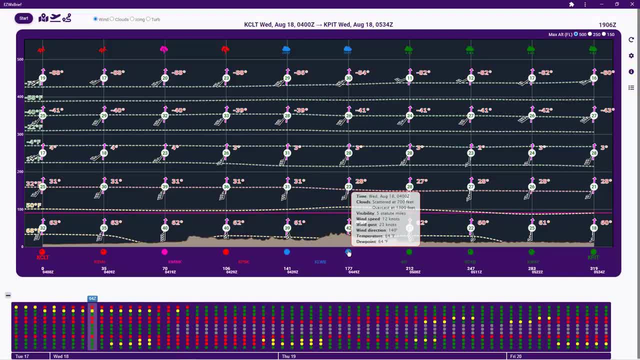 closest, essentially the closest whole hour in the recent past. So the 4Z forecast will persist all the way through And then, once you get beyond 5Z, that'll persist all the way through to 6Z. So in this case we end up at 0534 Zulu out of Pittsburgh. 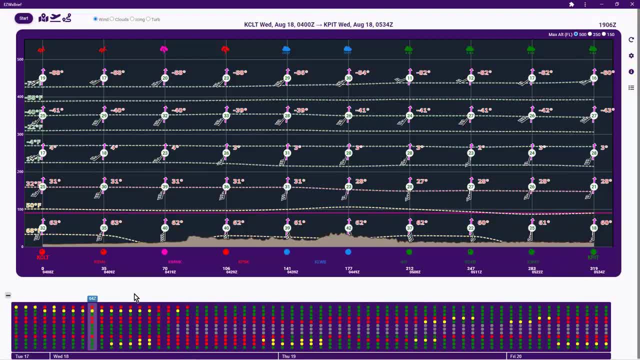 So it's going to use the 5Z forecast here. Moreover, the same thing happens with the personal minimum evaluation that's going on here as well, that if you're departing at 5Z, it knows that something is going to happen along. 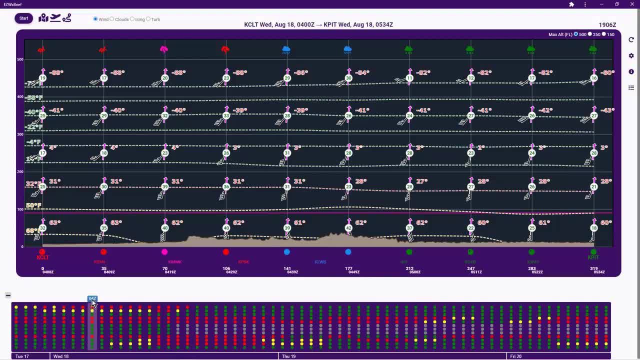 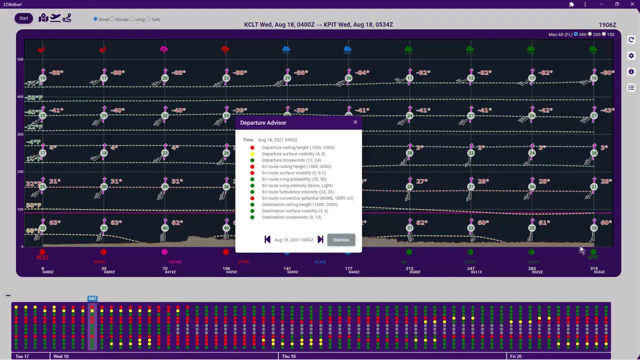 that route of flight by the time you get to that particular location. So it's able to make that determination in a way that it knows that, hey, if it's going to clear up by the time you get to your destination here, your destination ceiling height might be well within your range. 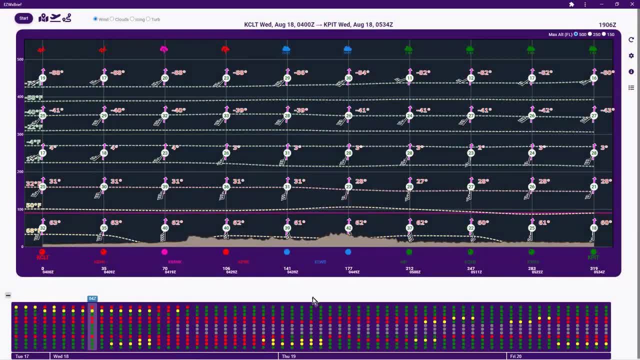 But, again, it knows how long it's going to take you to get there and it's evaluating all these dots, are evaluating things as you progress along the route of flight. So, again, if you were to be in a situation where you depart, 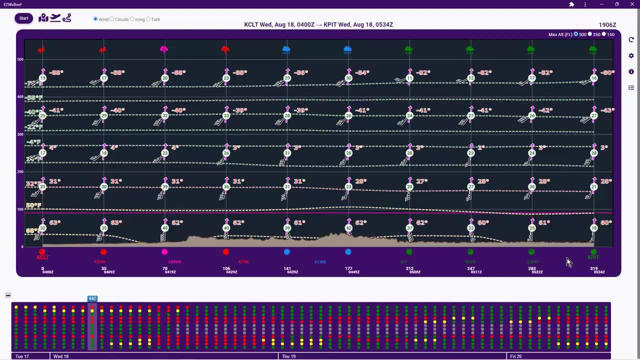 and, let's say, the weather is going to be really bad at your destination, but in the next hour or two it's going to improve again. the departure advisor will take all that into consideration. So now, all of the data that you see here, other than observational data, 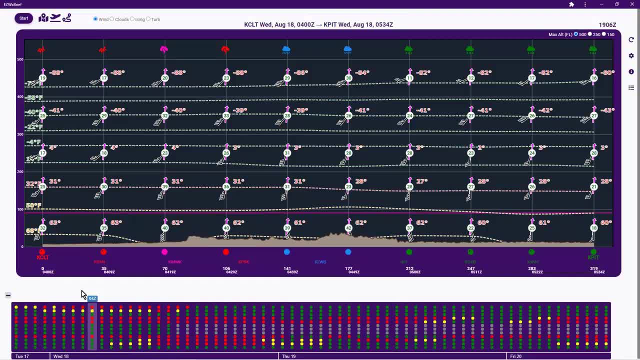 comes from a variety of different weather forecast models. Now, I'm not going to give you the specifics of each of these different elements in terms of what goes into that particular forecast that you see in EasyWeatherBrief, whether it's wind, temperature, icing, turbulence. 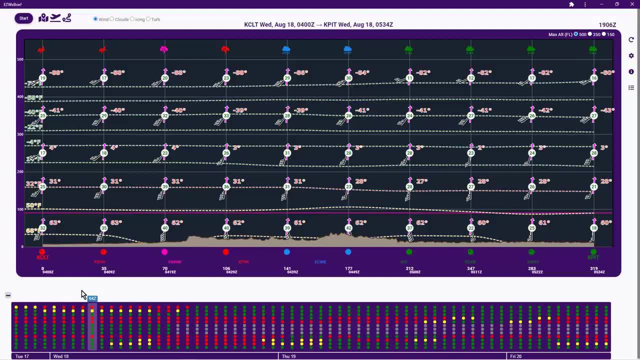 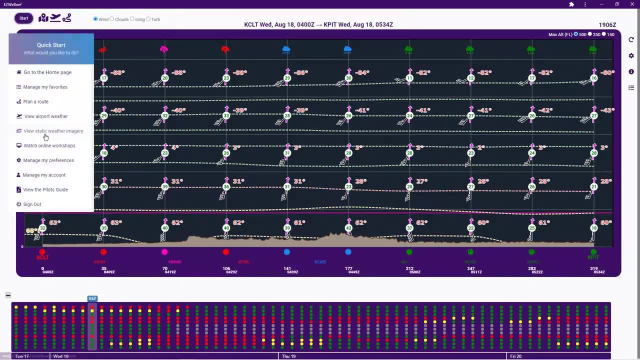 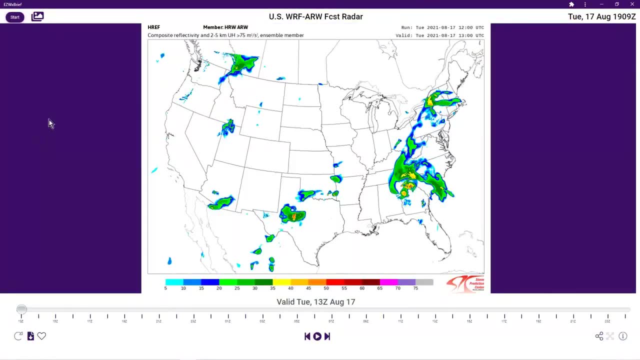 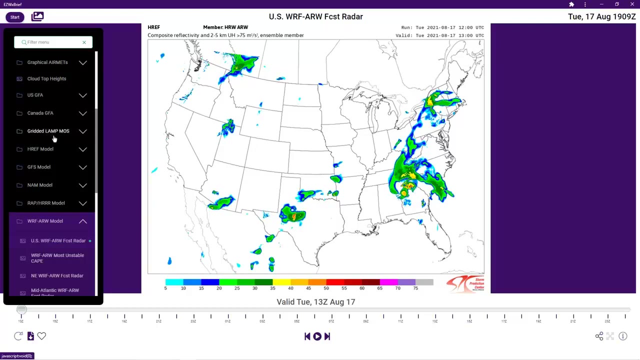 but it does come from a numerical weather prediction model. So let's go back and take a look at the imagery where you'll see most of the weather forecast models, and we'll start out with kind of an overview of the different forecast models that are available in EasyWeatherBrief. 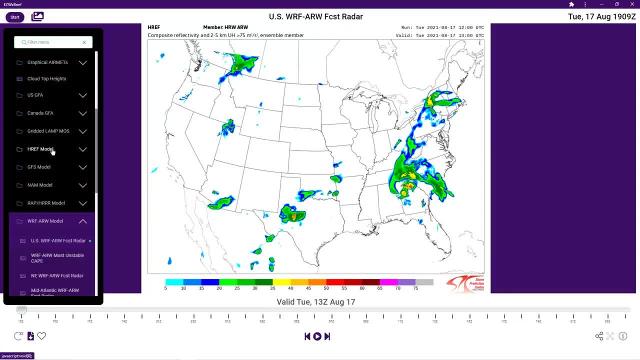 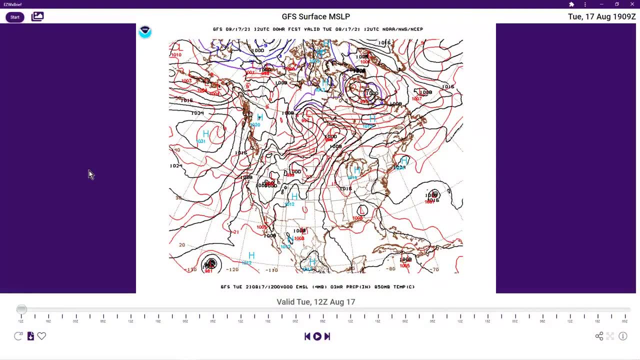 So let me just take one step here and we'll start out with the GFS model for now. but let's just take one step backwards and talk again about the basic elements to what we see in terms of data that we use for making decisions. 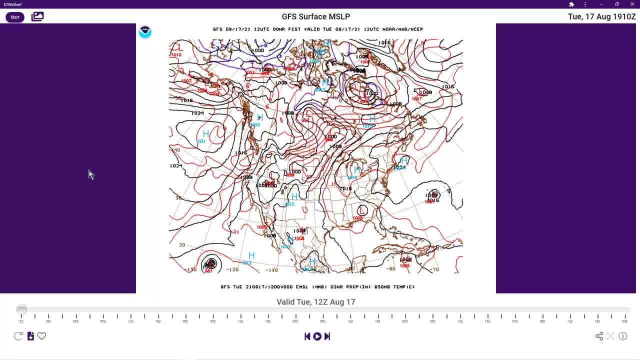 Okay, The first. you kind of categorize it into four- mostly three, but four different kind of categories. Well, the first category is observational data, That's from sensors, Things like if you were to listen to your AWOS or ASOS before you depart. 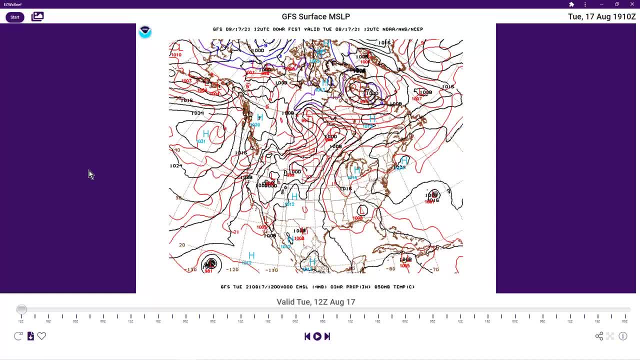 it's coming from various different sensors for wind and ceiling and visibility and such Observational data in the background. So, ultimately, you're talking about weather forecasts, you're talking about pilot weather reports, satellite imagery, a radar mosaic. All those are based from observational data. 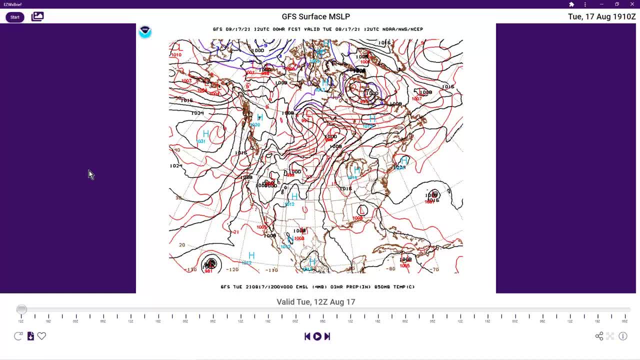 and they're valid always in the recent past. Then there are something essentially called analyses, which are always valid in the past and they can be generated by humans or they can be generated by forecast models or computers, And then you have basically forecasts that are always valid in the future. 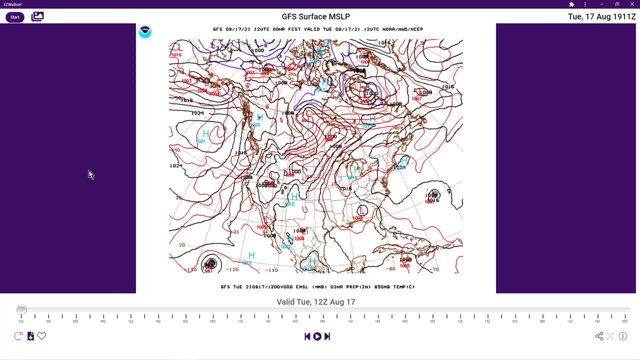 although if you stare at a forecast long enough, eventually time will pass that valid time that you're looking at. But in the end, forecasts are essentially for the future and they're always- well, I shouldn't say always- they are potentially generated by a human. 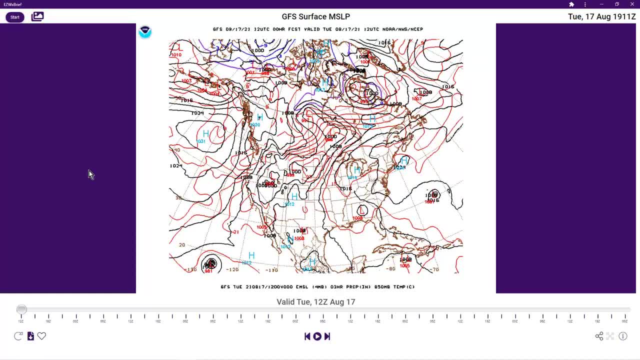 for instance, a prob chart, or they can be generated by a computer. A forecast model- Now one of the pet peeves of mine- and I hear this all the time- the forecast models are. all they are are just simple interpretations. 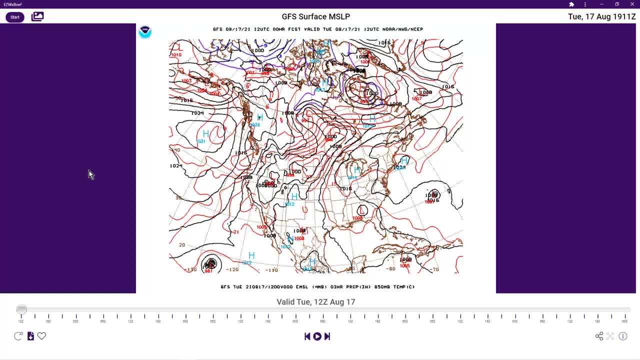 or I'm going to say interpolations of the radio signs that are launched every 12 hours And that couldn't be further from the truth. Forecast models ingest that data and we don't have a lot of data over the oceans. we certainly don't have radio signs. 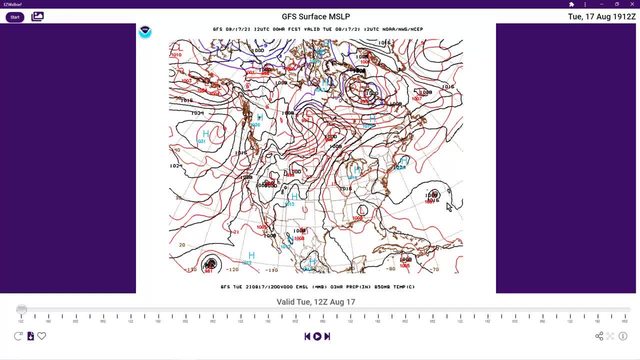 they're essentially sent up, or weather balloons over the oceans. but that data does go into the forecast models that we'll talk about. but there's other data: surface observations, aircraft reports from commercial airliners. there's satellite data that they use. 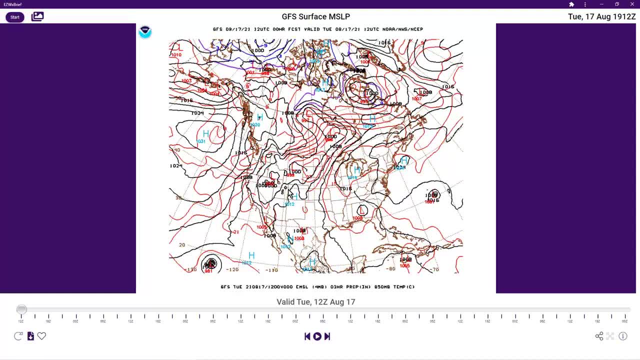 sea surface temperatures, soil moisture, All those kind of elements are observational data that gets generated and eventually ingested into these forecast models. and the forecast models are pretty sophisticated computer programs that take all that data, run it through the equations of motion, basically physical and thermodynamic equations. 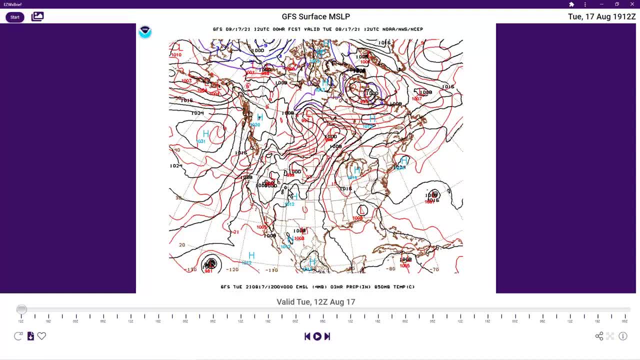 and that eventually produces some kind of solution. We call that a forecast, And that forecast model essentially is something that meteorologists will have to interpret. Well, it turns out that that forecast information that comes from these models is also very interesting to us as well. 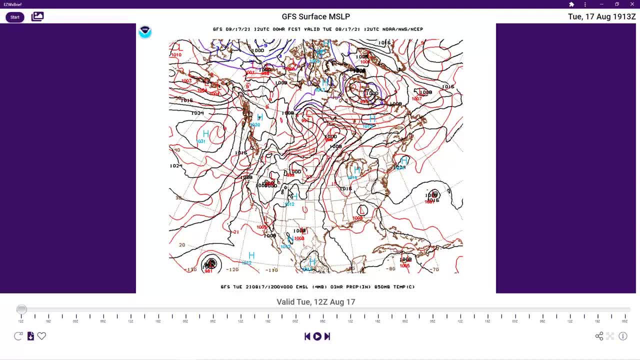 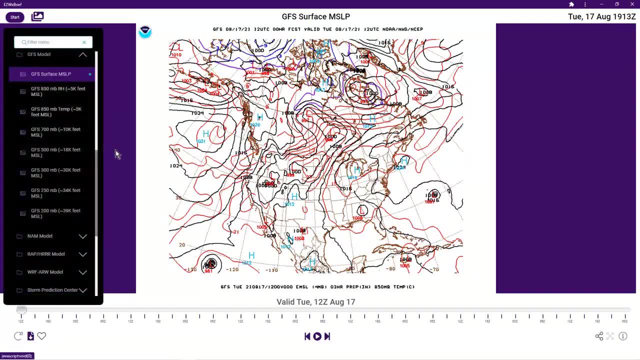 if you want to make use of it, And that's what I'm going to try to talk about today. So there are, generally speaking, dozens of forecast models out there: Forecasts from the National Weather Service, forecasts from Canada. there's forecasts from the European Center for Media Range Forecasting. 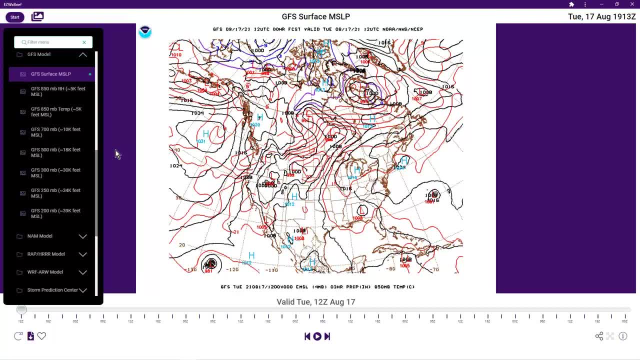 some of the military, like the Navy, has their own model. So there's lots of different forecast models out there and most meteorologists have access to all of those models when they produce their forecasts- Not that they use every single model to produce a forecast. 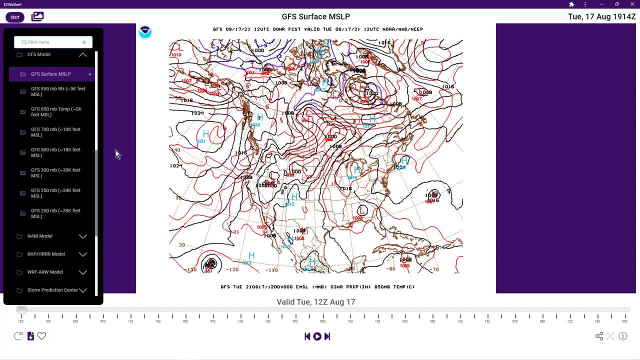 but they do Normally. they look at the models to see how well they're doing and they pick a model, or they may do a blend of multiple models to produce a forecast for a Prague chart, for instance, or a terminal forecast. 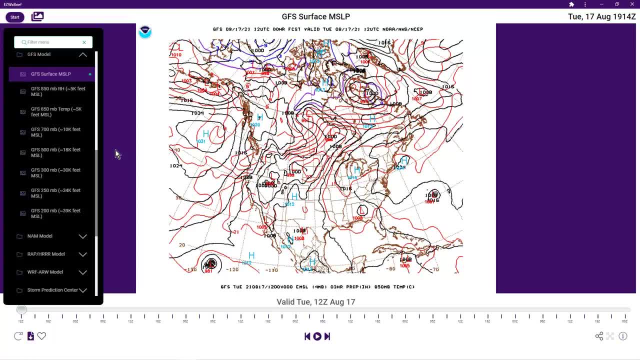 But the National Weather Service also pushes out a lot of this information, and also the European Center, the Canadians, all those push out their forecasts so that you and I could essentially look at them And interpret them, if you know and understand what they're telling you. 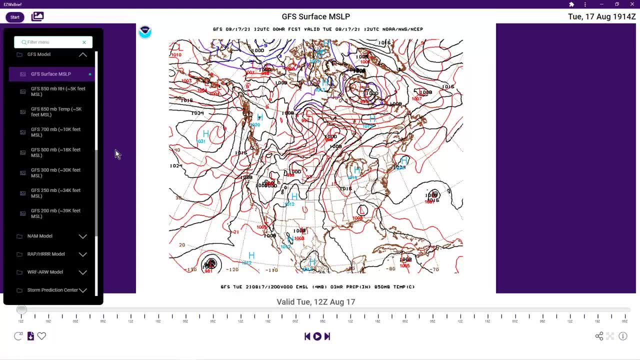 Now, some of this may be a little bit too extreme for most pilots and I don't want to go into that, but there's a lot of good information that can come out of these forecast models if you spend some time learning how to interpret it. 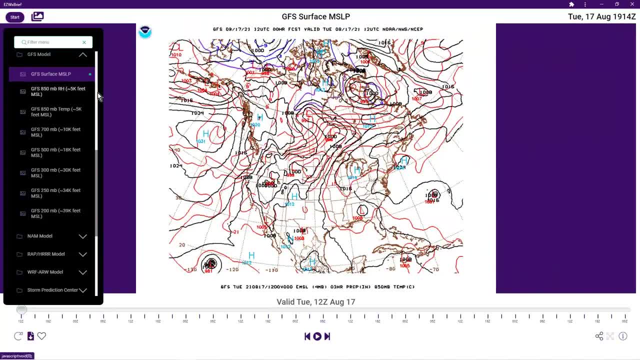 So first of all let's talk about the kind of the general aspect of these forecast models. There are multiple forecast models the National Weather Service puts out And, for the most part, Easy Weather Brief focuses on those particular models. They generally are looking at it from a standpoint of 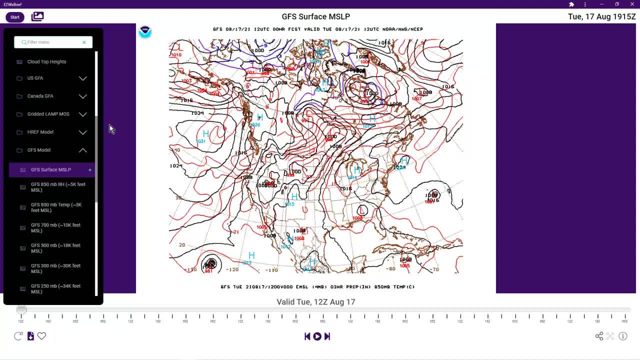 there's a global model, then we have a kind of a North American model and then we have a usually a rapid refresh model, a model that is run more frequently. So the global model has a global domain. It forecasts for everywhere around the globe. 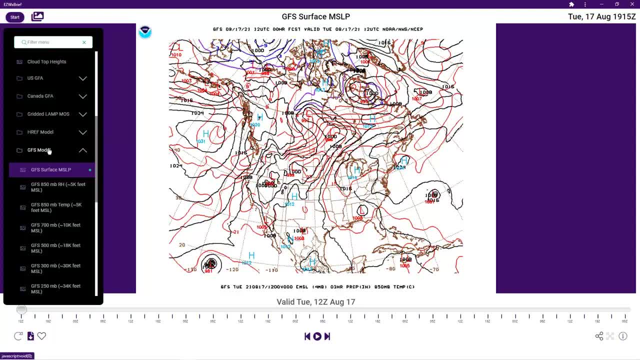 And the one that's used in Easy Weather Brief is called the GFS model- Global Forecast System Model- And this has its some of its early days back in aviation. In fact, there was a model when I was working as a National Weather Service. 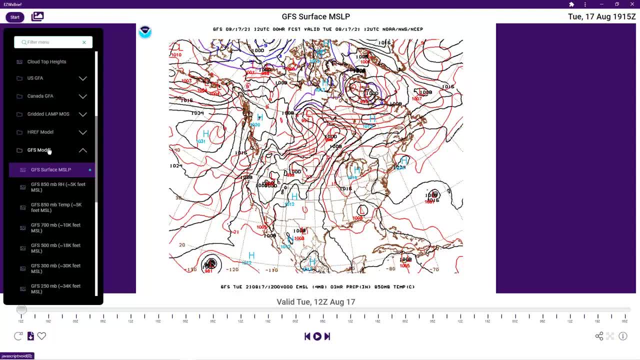 research meteorologist called the Aviation Model, And most of the forecasting that you see now from a numerical weather prediction standpoint was all primarily for aviation, to support aircraft going from point A to point B and understanding what the winds aloft are and what the general forecast was. 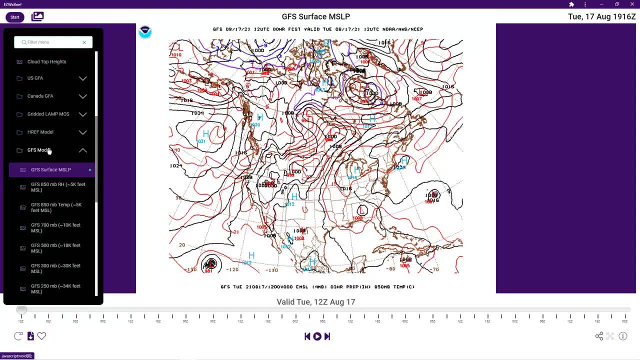 And so out of that eventually grew the GFS model, And they've made many, many updates to it over the years to improve it. as we get better forecasting, more significant computers to be able to do some of the number crunching, Then we can actually provide a much better forecast. 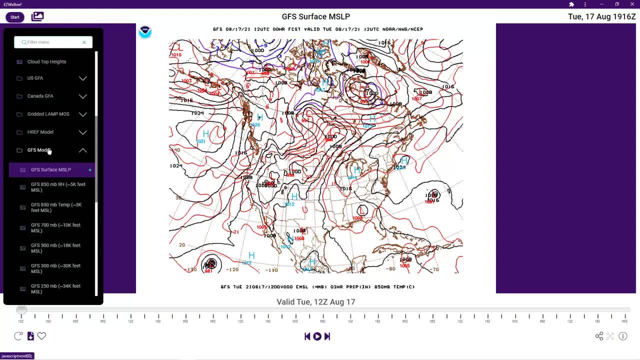 And that's again over the years has gotten much, much better. So the GFS model is a global model And you see it here. It's just showing you essentially what's happening over the entire area of North America. There's also the North American model. 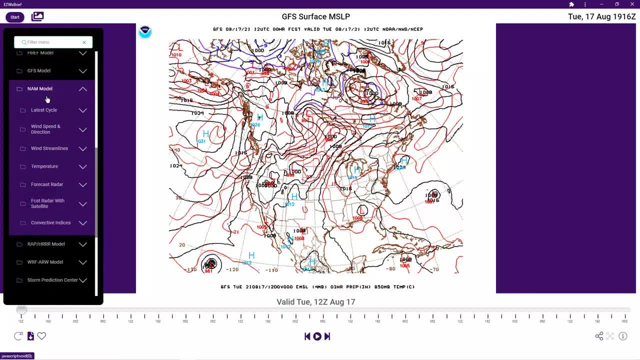 which is called the North American model or the North American mesoscale model. It's also in this particular case, it's also run by the National Weather Service, but it has a North American domain associated with it. Then there's the rapid refresh. 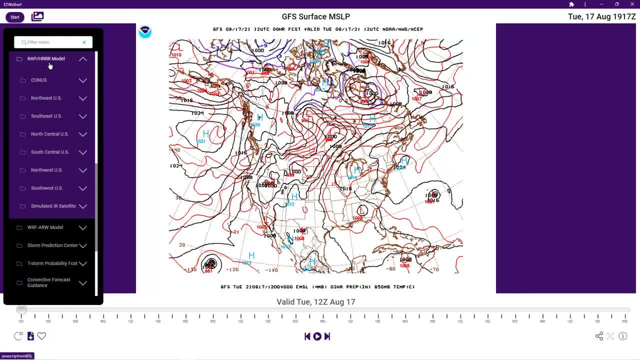 or high resolution rapid refresh, the HER model. that also has a kind of a North American domain as well. But the different characteristics of each model certainly provide a different view of what may be happening with respect to the weather. So the global forecast system does really well. 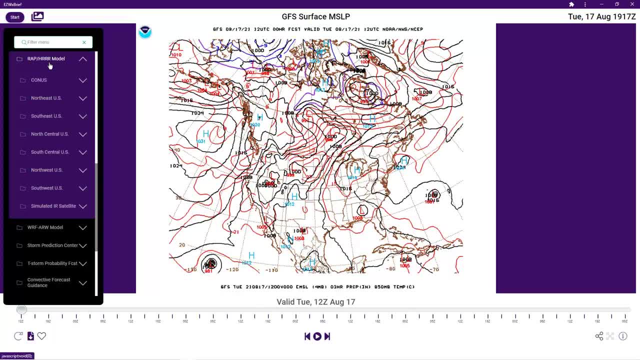 at showing the overall upper weather flow patterns- And that's important to understand because ultimately that's where most aviation flies- up at flight level 390. And understanding what the wind patterns are up there. and the simple fact is it's a very high resolution model vertically. 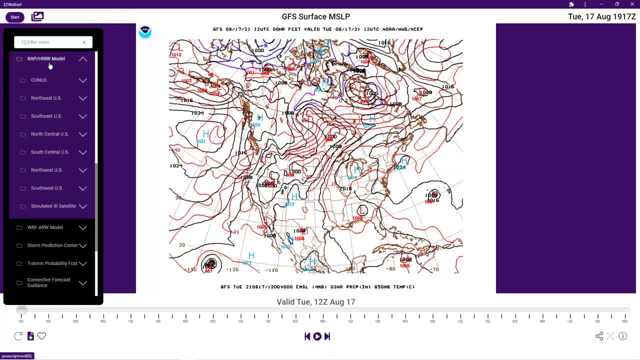 better than the other models, So it does extremely well at predicting these main upper level patterns, Whereas in this particular case it's run every six hours. So that's 12Z, 18Z, 0Z and 6Z. 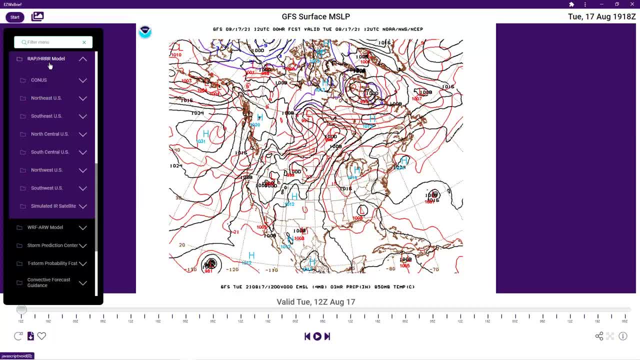 It actually is not run exactly at those times, but usually somewhere around three to four hours later than that, as it's doing what's called data assimilation, bringing all the data in, Whereas the North American mesoscale model also gets updated or gets rerun every six hours as well. 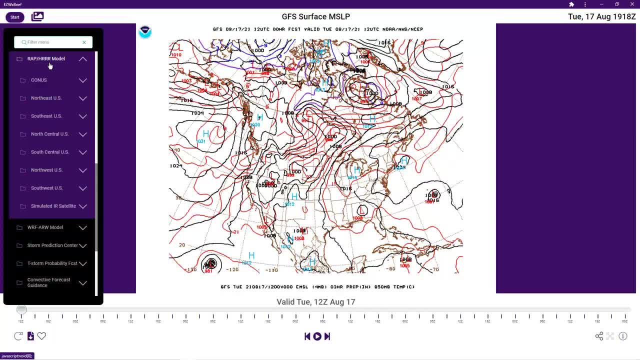 Its time when it starts is usually about an hour and a half after that time. So the 12Z run of the model usually starts its run time around 1330 Zulu. And then you have the high resolution rapid refresh model which gets run every single hour. 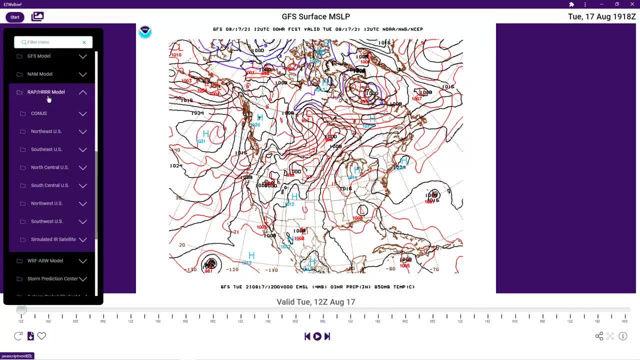 Hence the term rapid refresh, And the high resolution version of it is literally that It's a high resolution kind of over the continental United States. Now the global forecast system makes a forecast out to 16 days in the future, Whereas the North American mesoscale model goes out to three and a half hours. 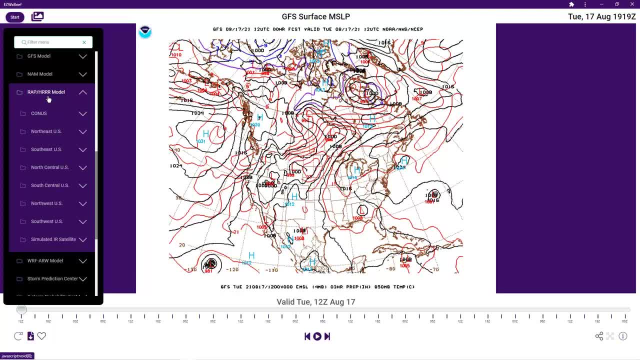 Three and a half days or 84 hours, And the rapid refresh model now seems like it changes all the time, but essentially is a model that goes out just beyond a little bit beyond 24 hours, In some cases out even as far as 38 hours. 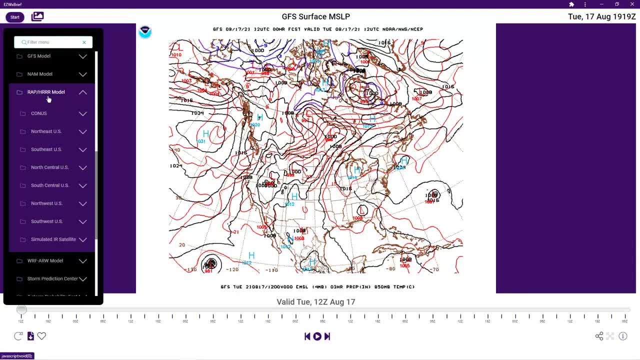 So in the end, the nice thing about the rapid refresh model is that it gets updated every single hour, So as the weather is changing and the models essentially can then adapt to the changing weather, And usually the rapid refresh is a good model to use, let's say, the day of your flight. 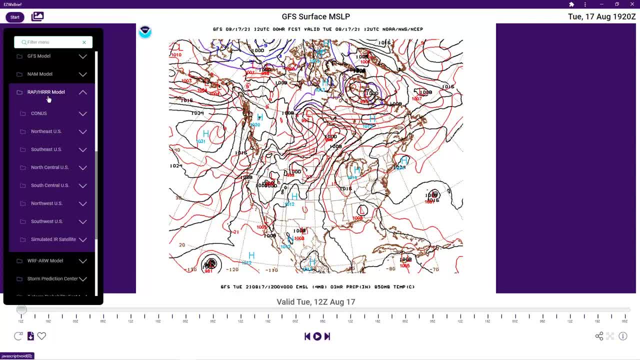 Whereas if you're looking at the longer range forecast, the North American mesoscale or GFS model might be better for that two to three to four day range beyond your time essentially when you're going to depart. So those are all different kind of high level views of things. 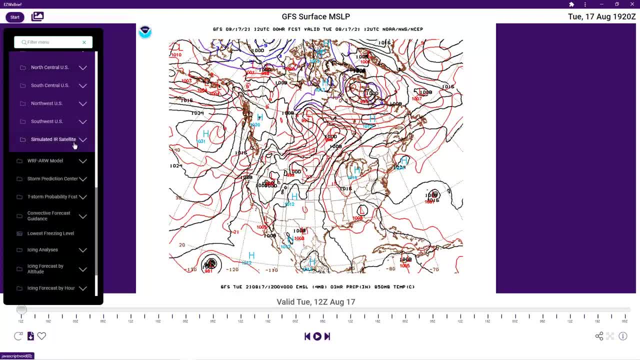 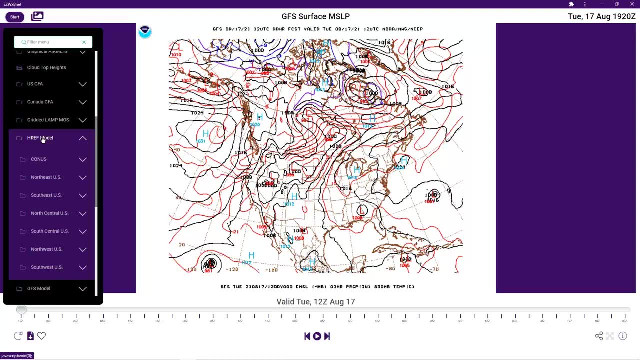 There are also kind of variants to this, and that is you'll see other models that are provided in EasyWeatherBrief. One of those is this HREF model, or high resolution ensemble forecast. So another approach to forecasting is you can rerun the forecast model multiple times. 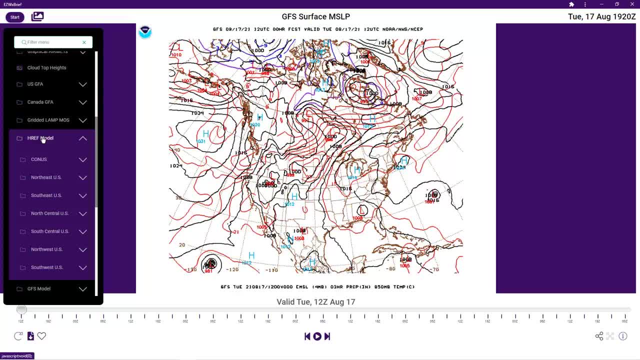 and you can essentially tweak the initial conditions just a little bit for each run and you exactly examine what happens to that particular forecast. So if the forecast is, if the initial conditions are tweaked just a little bit and you get a totally different forecast, then the model is very sensitive to those initial conditions. 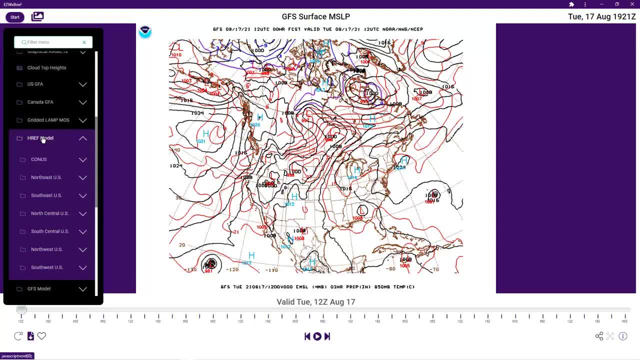 and therefore the certainty of that forecast may go way down. So forecasters can tell whether or not there's really some major issues with these certain runs of the models based on how the model responds to each one of those runs, and we call that an ensemble. 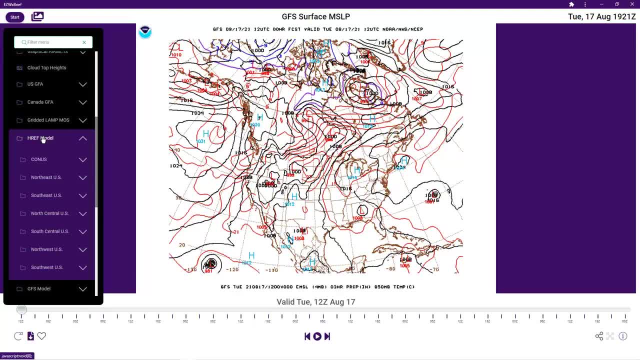 You've probably seen the spaghetti diagrams with hurricanes and such as they come on and some have some really wild tracks and others essentially are very much outliers. but the forecasters are looking at the National Hurricane Center, kind of looking at where that mean is and understanding kind of what models do well in certain situations. 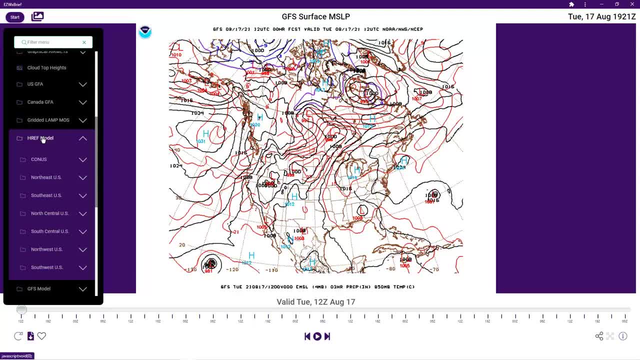 and then they can produce a much better forecast. But when all those tracks kind of line up, it's a good indication that there's a lot of high confidence in that. So ensemble models do an extremely good job for the most part from that standpoint. 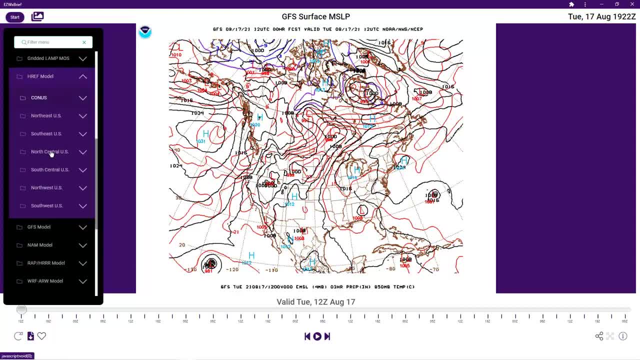 So the HREF model- High Resolution Ensemble Forecast- is a model I like a lot. Now, each of these models has different information associated with it. For instance, you can see the GFS has a 850 millibar, 700 millibar. 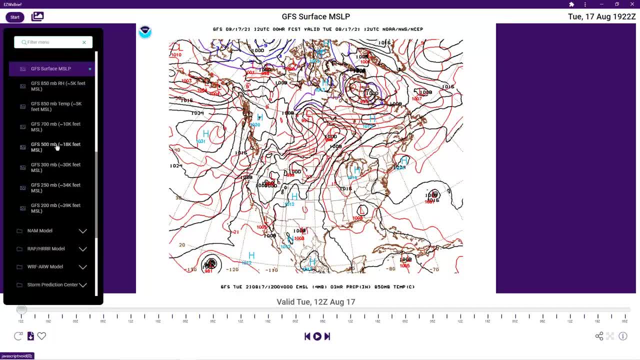 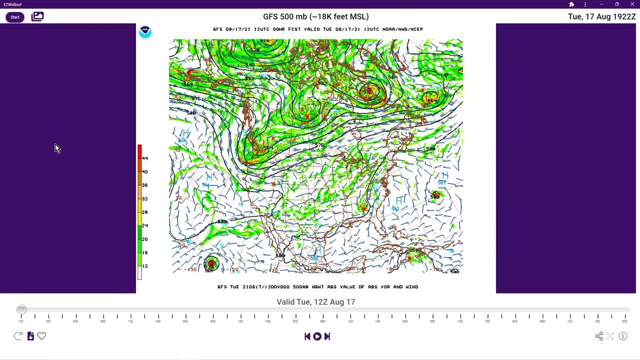 500 millibar, 300,, 250, and then 200.. So you can look at any one of these particular levels. Again, I'm not going to be able to spend a lot of time going through this particular element here. 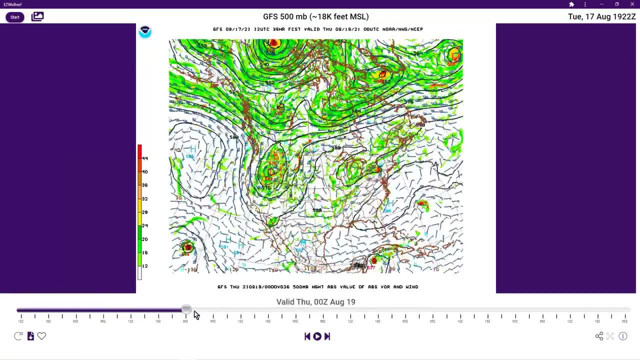 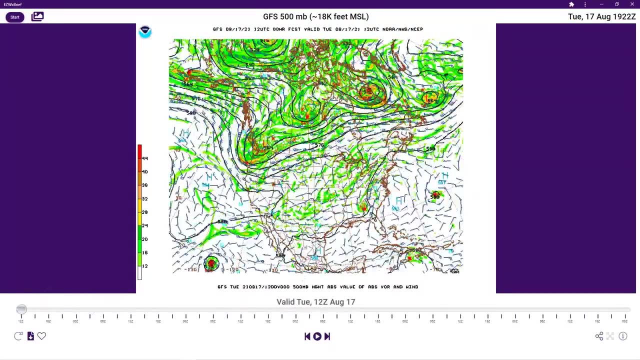 But in general you can kind of start to see the pattern that this is at 500 millibars of what's happening in the atmosphere, And it also even gives you the ability to see kind of: there's this tropical system, Fred, that came on shore. 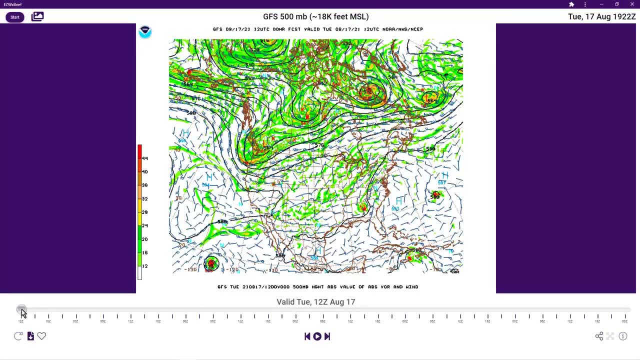 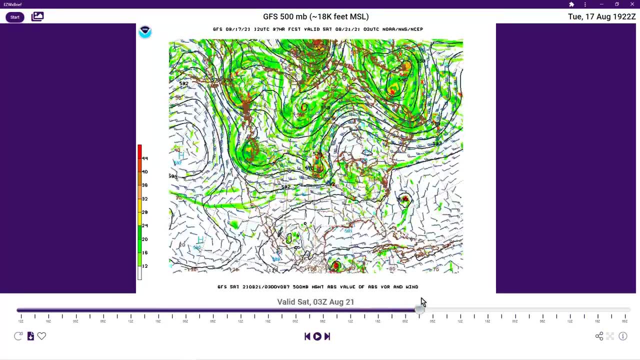 here along the Gulf Coast And you can see Grace at the bottom making its way just the south of Cuba, over the Yucatan Peninsula and eventually into Mexico. So it can give you a lot of good information about what's happening at the upper levels. 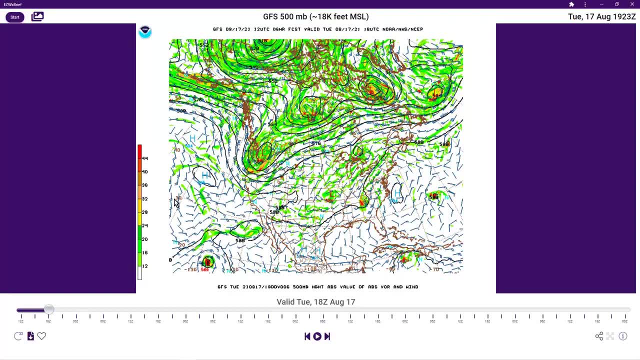 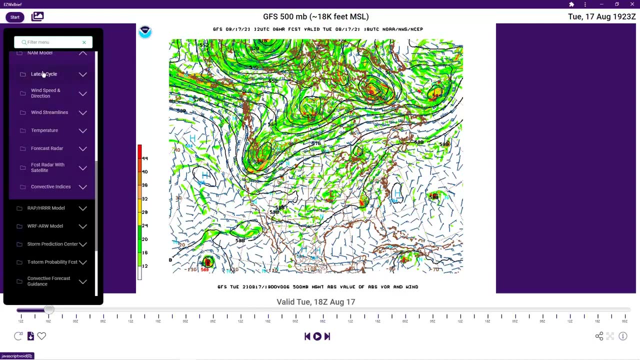 But that can then equate to understanding where the most significant weather is occurring when you look at these upper level troughs and ridges and such, And then each one of the models has all that same kind of information. For the NAM. you can go to the latest cycle. 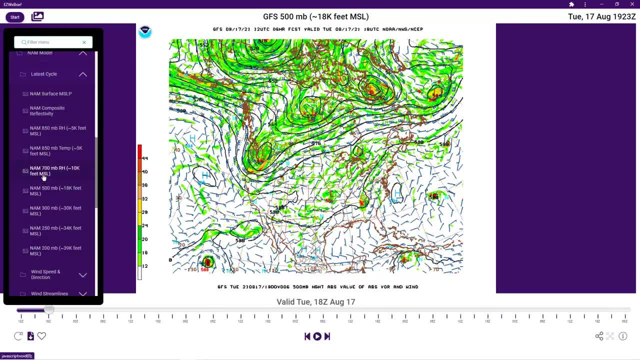 and see all those charts. But there are other charts as well. You can also look at the, let's say, the forecast radar from the NAM. So we want to kind of look at what's going to happen and we pretend that this is a 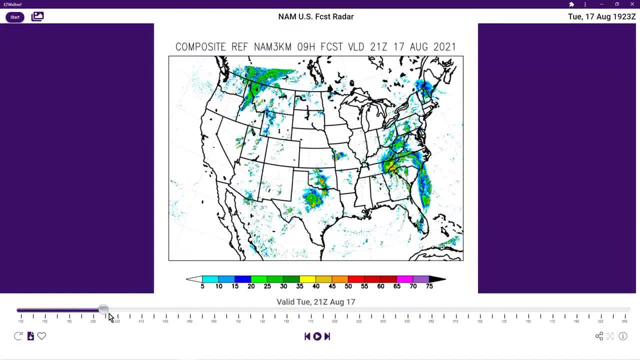 NEXRAD image in the future. So this is a forecast, but it's looking at a NEXRAD image in the future and kind of give you a better understanding of how weather systems are going to evolve in a way that makes a lot more sense to us as pilots. 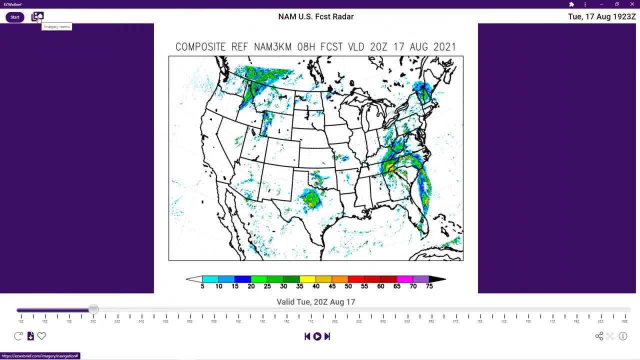 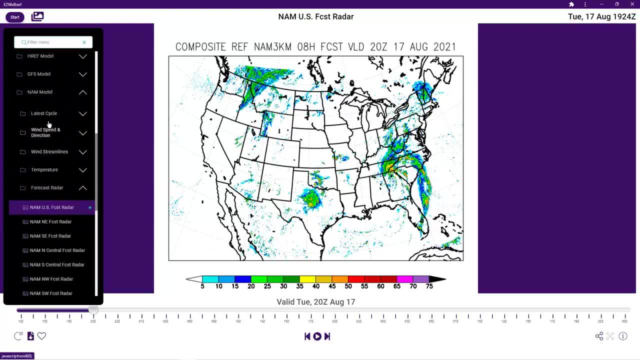 so we can kind of see what's happening there. And there are many other selections for the various different things, such as, if you wanted to see, let's say, the wind speed and direction, wind barbs at, let's say, 18,000 feet. 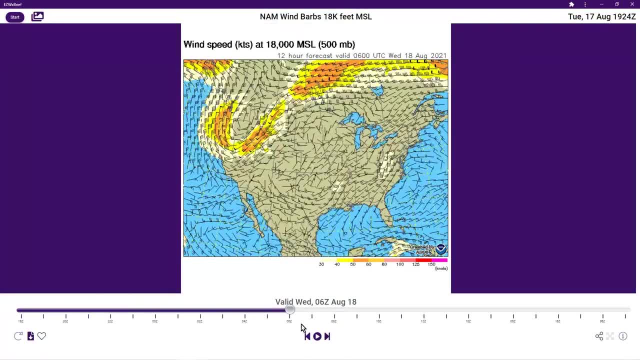 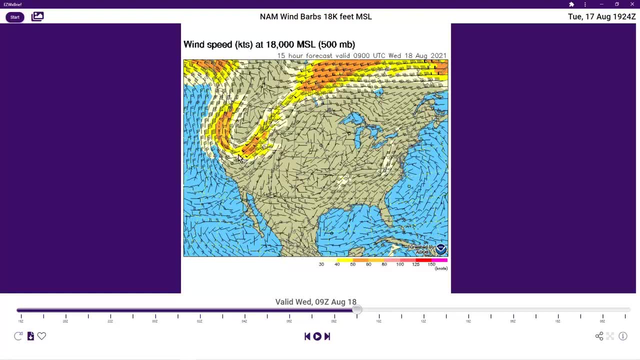 You can kind of see that how that evolves over time And again. this is going to show you the same kind of situation. There's a big upper level trough here. This is at 18,000 feet, But you see the wind barbs. 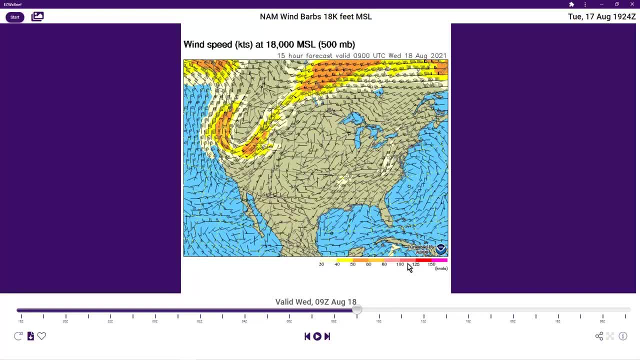 this again a little bit different. They color code it according to the strength of the wind, so the wind speeds. So anywhere you see the yellow here, it would be 40 to 50 knots. So that's all available and these all come from. 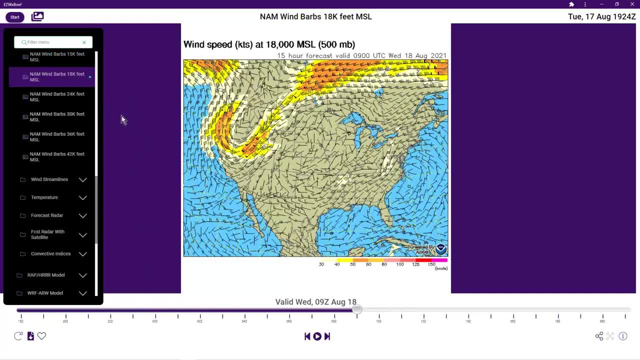 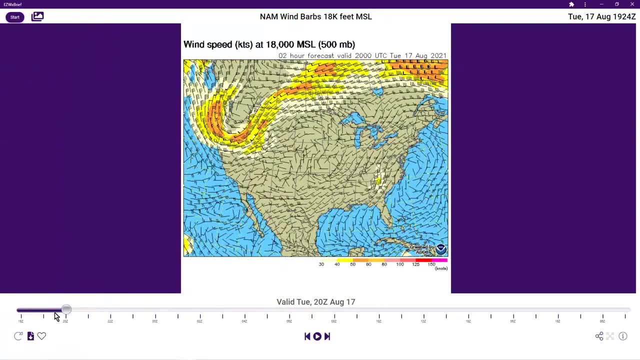 the numerical weather prediction model, The first, the way this works here, even though it says it's under the NAM, ultimately the first. the first sets here that you see are, you can see, are kind of an hourly hour by hour basis. 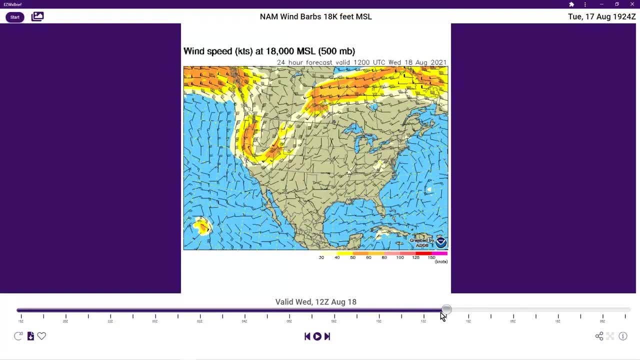 And eventually it kind of jumps to there we go. you can see it kind of change right there What jumps to 24 or every six hours, and that comes from the NAM itself. So the very first part of this is from the actual rapid refresh model. 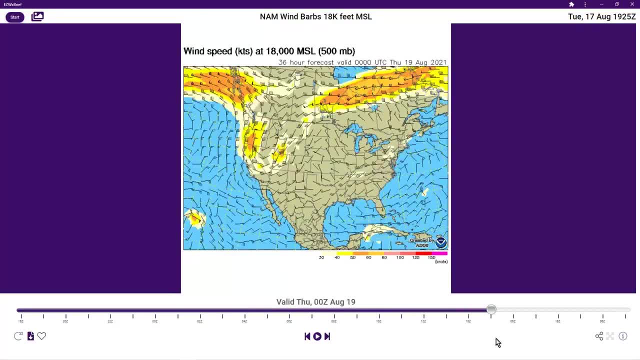 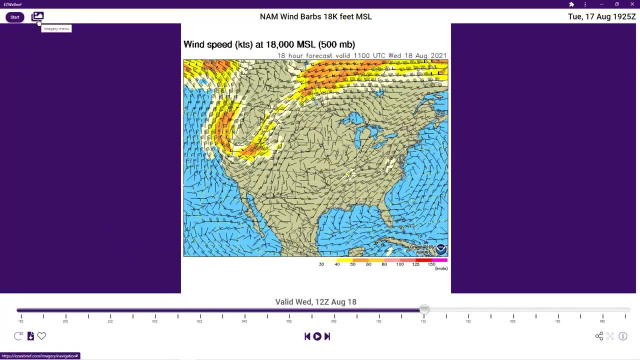 and then eventually it jumps to the NAM. I just decided to put them all together in one loop here rather than trying to spend a lot of time having to jump back and forth between the two. So I put them all under the North American mesoscale model here. 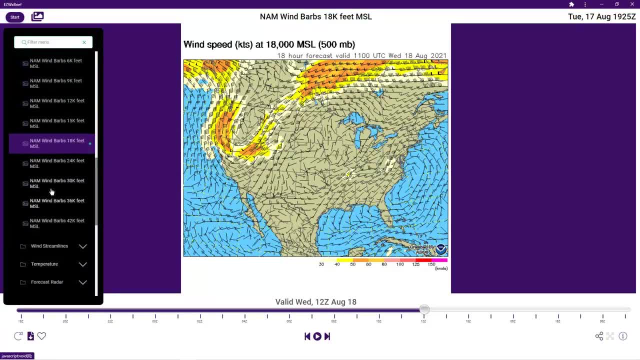 But you can also look at wind streamlines, temperature and such as far as that goes. So it's a lot of information at your fingertips using this imagery from a forecast model. Then there are kind of other aspects to this where they can put together different flavors. 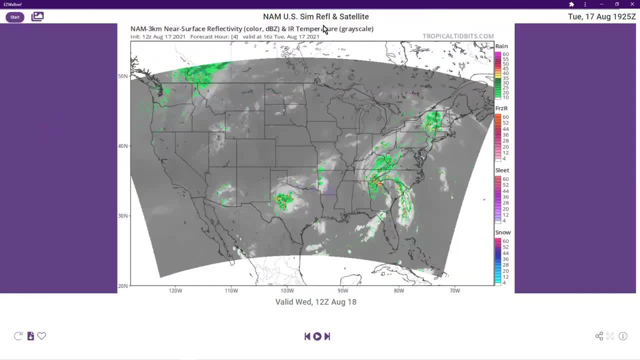 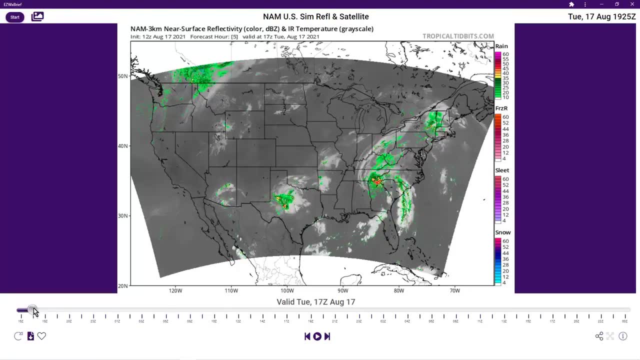 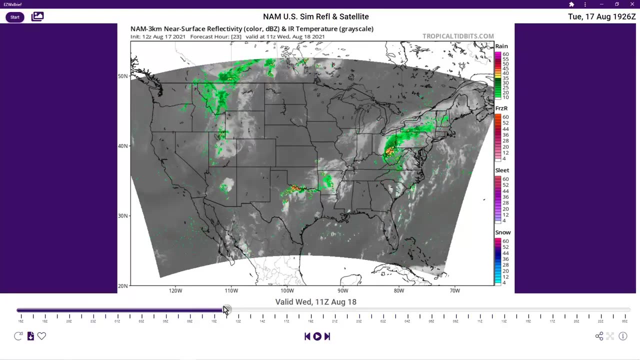 of forecast information. In this case this is from the simulate reflectivity, very similar to what we just saw, and satellite information. So anywhere you see the gray coloring, essentially this is the cloud depiction- forecast cloud depiction that might occur, And so the brighter white colors are those 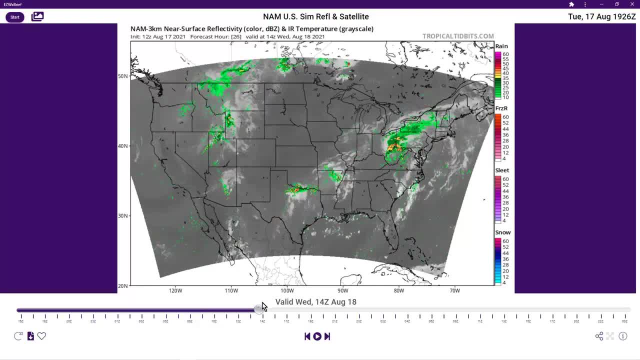 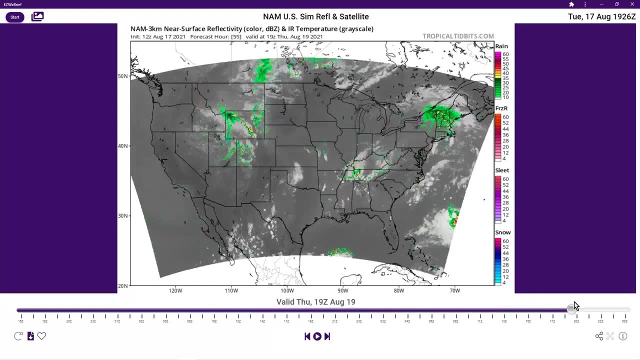 that are basically colder cloud top temperatures, which usually means we're dealing with higher temperatures or higher clouds- I should say colder temperatures- And it also overlays, in this particular case, the simulated reflectivity or forecast radar, and this goes out pretty far in the future overall. 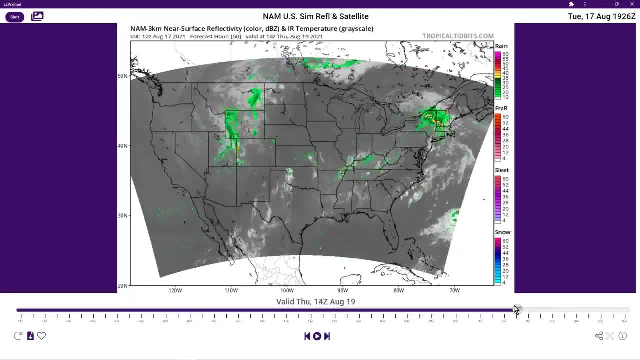 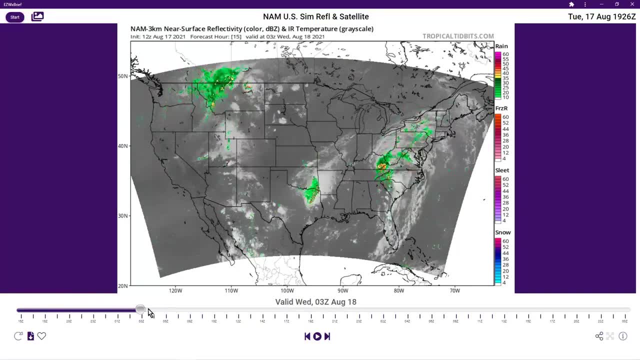 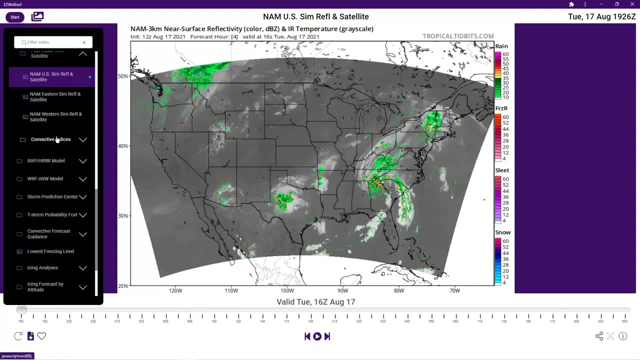 We're talking about 60 hour forecasts, so that gives you a really good understanding of what's happening over the next day or two in terms of how all this weather is going to evolve here And then you can also look at various different convective indices. 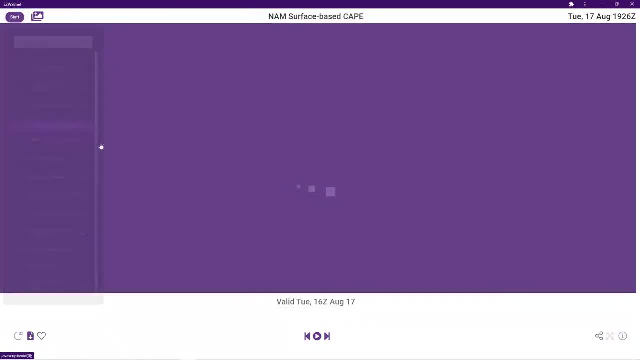 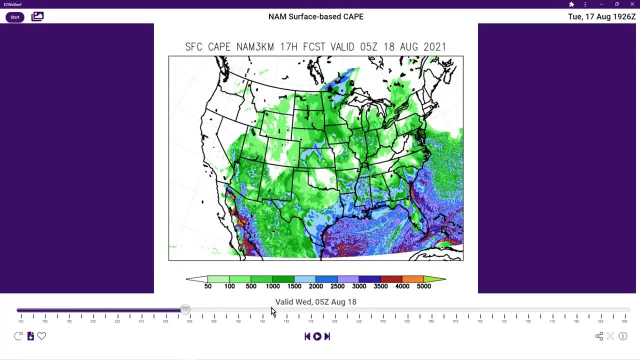 For instance, if you look at the surface base CAPE convective available potential energy, you could do that as well here. So you can see how the CAPE values anywhere. you would see the blues and purples and such. we have lots of high CAPE values there. 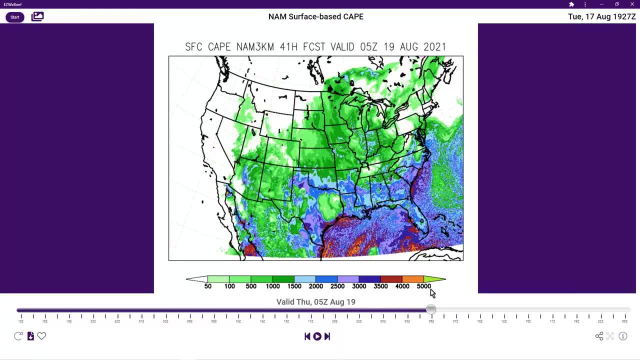 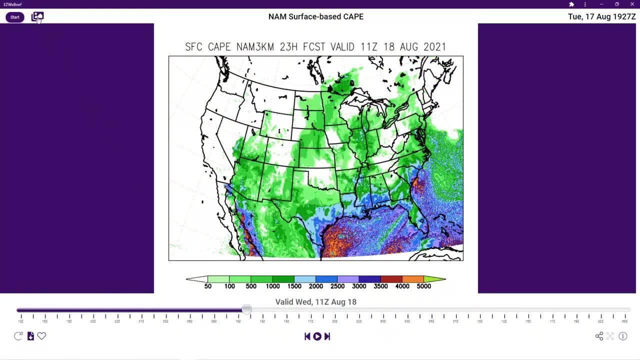 It doesn't necessarily mean thunderstorms. it just means you have ample instability in the atmosphere, ample moisture, And you could also look at this WRF ARRW model. This is also from the high resolution Ensemble forecast and once again, it gives you good information about. 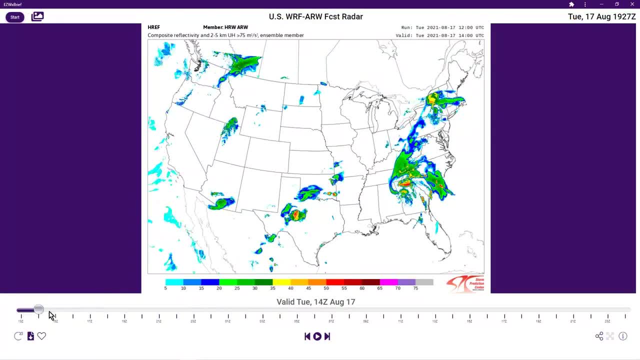 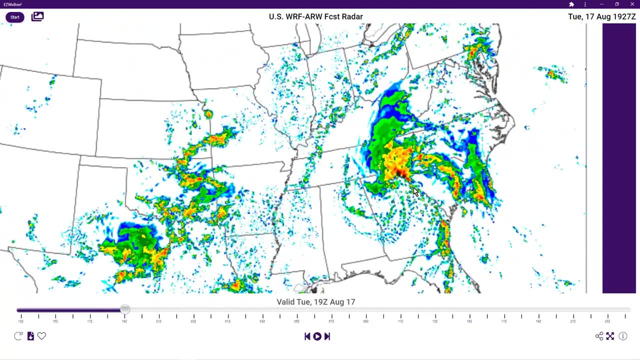 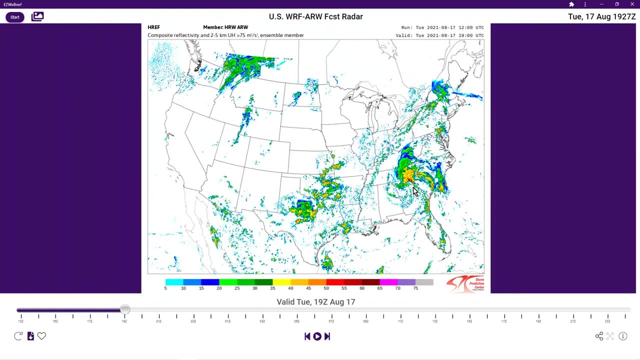 forecast radar depictions. This is probably one of my favorites here. The only big difference to this is that this is only run twice a day and it's at 0 and 12Z, and because it's not monitored by the National Weather Service. 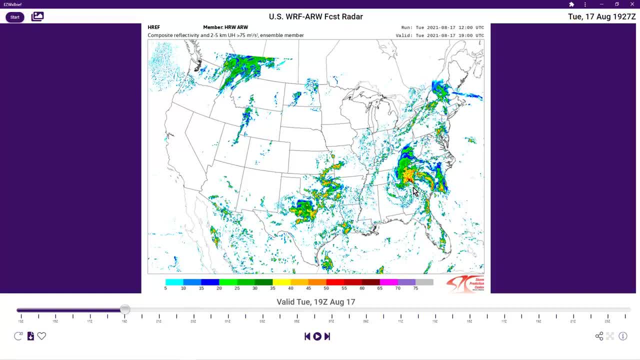 you're not going to see this right off the bat after 12Z. Instead, it's going to take usually five or six hours after that time. So when you wake up in the morning, the latest one at, say, 12Z- you're going to actually be using the 0Z. 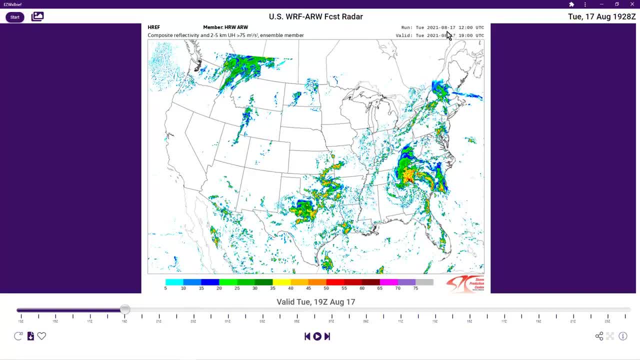 from the previous run, So this is the latest here. 12Z. You see that up here on the chart and I always like to double check the time that we put here. This is put in by Easy Weather Brief. Sometimes we guess right. 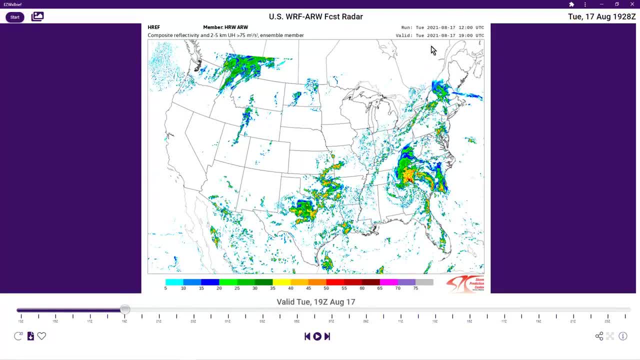 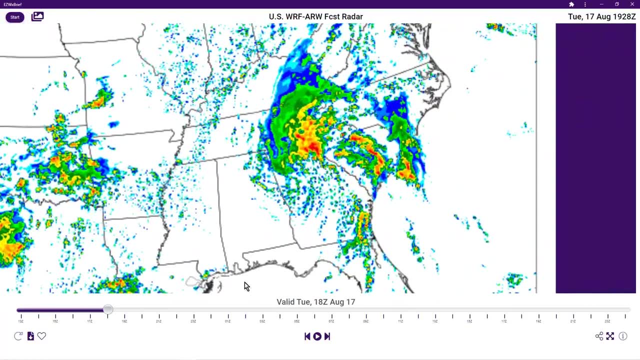 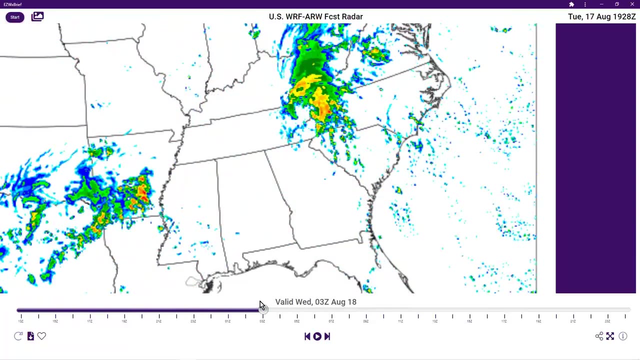 other times we don't. So you always want to compare that accordingly. But this again gives you a better indication of kind of how the weather system is going to evolve over time and give you a little better indication of whether or not this is going to meet your specific. 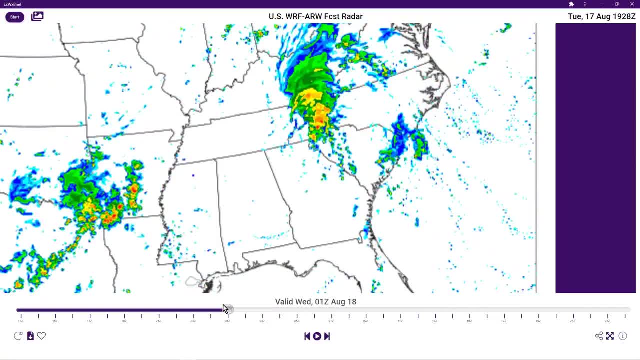 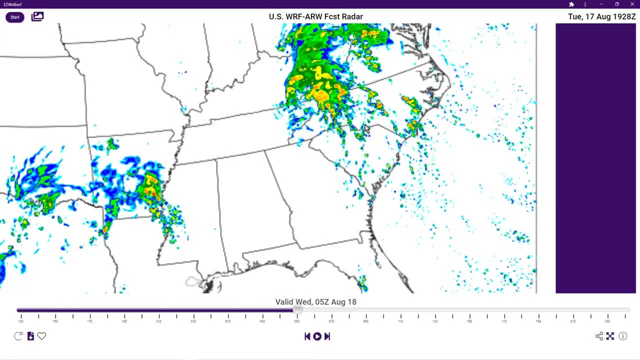 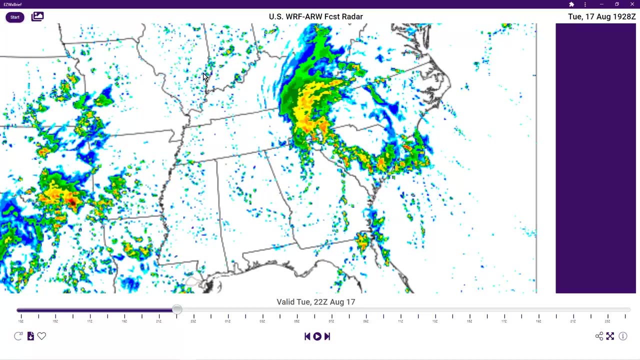 risk tolerances. If you're totally adverse to any kind of convective element, you definitely don't want to be flying today in the Mid-Atlantic and part of the Southeast, But for the most part most of the Gulf Coast states, all the way up through into 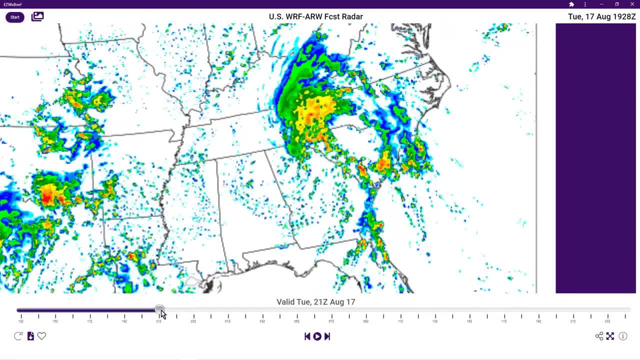 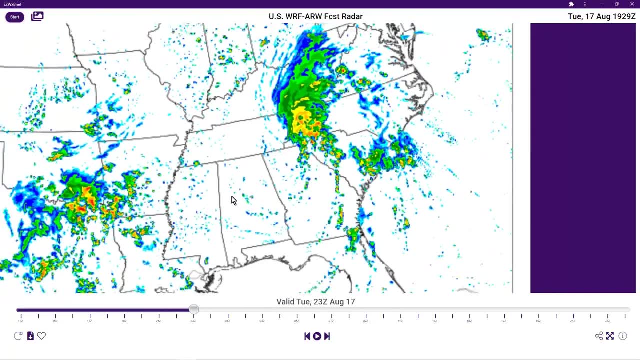 Middle Mississippi Valley and such doesn't look too bad. if you're flying later this afternoon into the early evening, It tends to look really well. So this gives you again a very quick analysis and it's in a way that makes a lot of sense for you as a pilot. 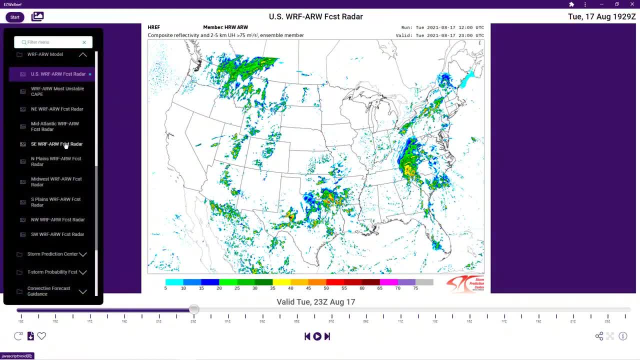 of how it all comes together. Once again, there are a lot of other different things that you can pull from these various different models. There is a limited set of data that we provide in Easy Weather Brief, but you can also get a lot of this information. 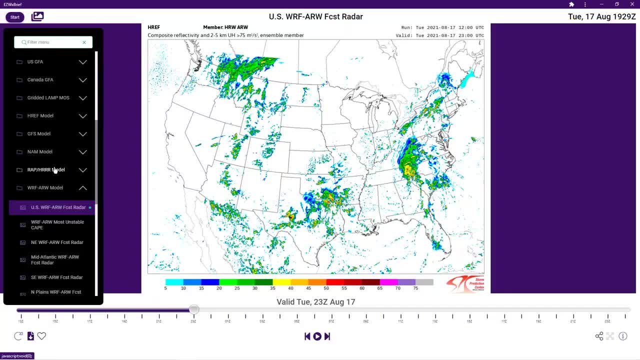 out at the National Centers for Environmental Prediction if you wanted to go specifically to the source where I pull it from. But for the most part you're going to find that this is kind of the stuff that makes the kind of the best information for pilots. 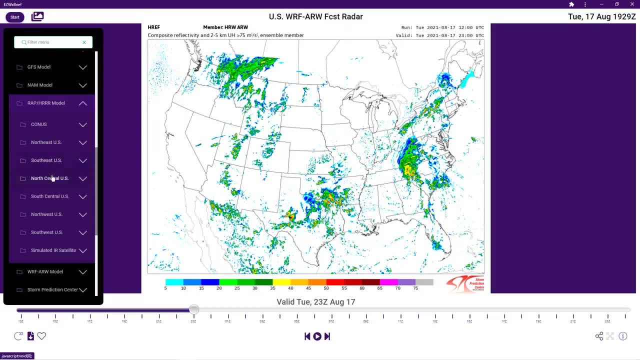 So I kind of pull all this together And you know things like, you'll find that you'll get really high resolution information from some of these models. For instance, I can go to the southeast US and go to the forecast radar there. 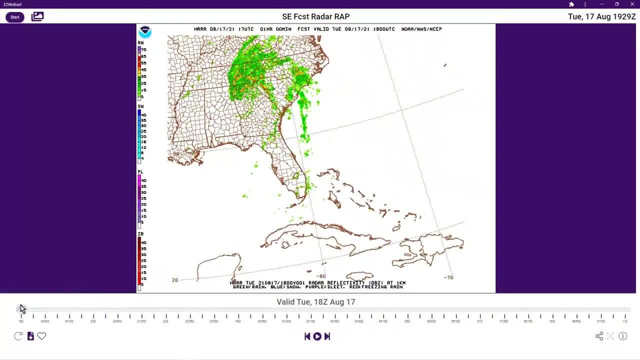 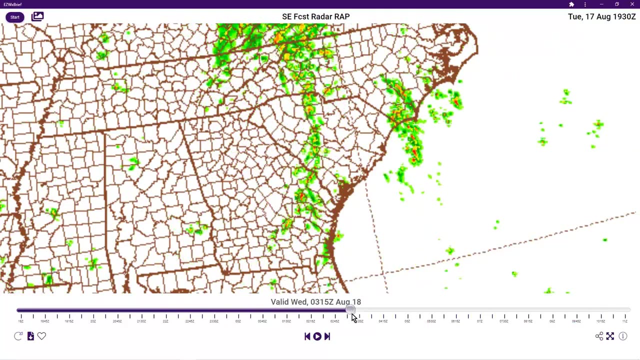 The neat thing about this particular chart is that this, every single kind of movement here, is a 15-minute time step. So you've got a lot of resolution time steps. You've got a lot of resolution time-wise, in seeing how all this is going to evolve over time. 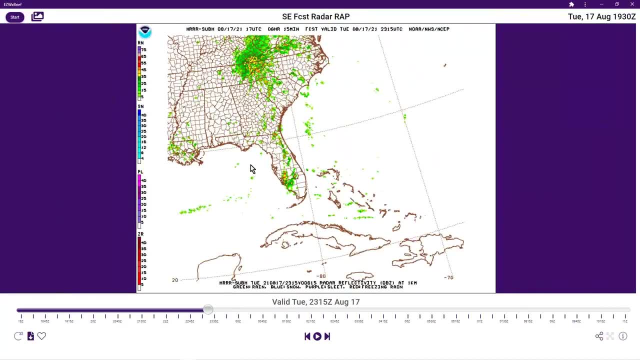 But again, this is a simulated reflectivity. that happens to be what we see here. You read some of the details at the bottom, at one kilometer up. So it's basically suggesting that at one kilometer above the surface is where this is kind of being forecast from. 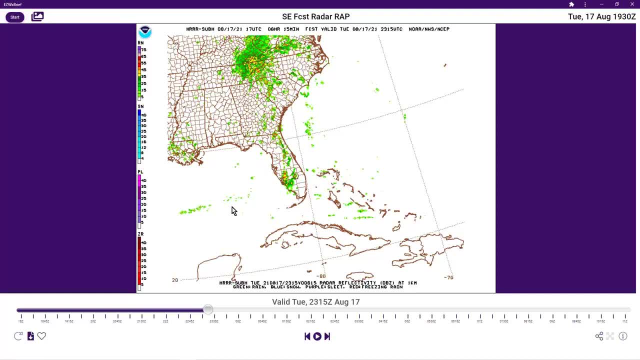 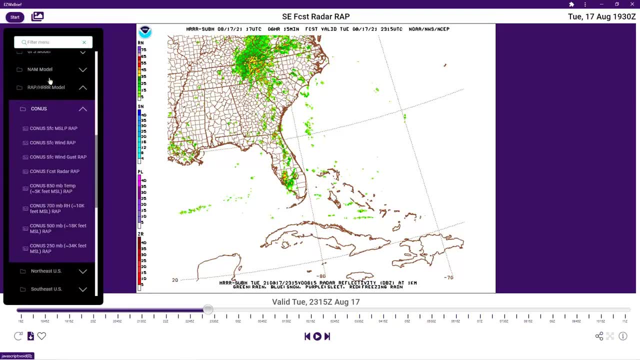 So I always look at that as kind of what's falling out of the base of the cloud, so to speak. So I would encourage you to play around with the various different forecast models and pick and choose And remember you can actually go at some point in time. 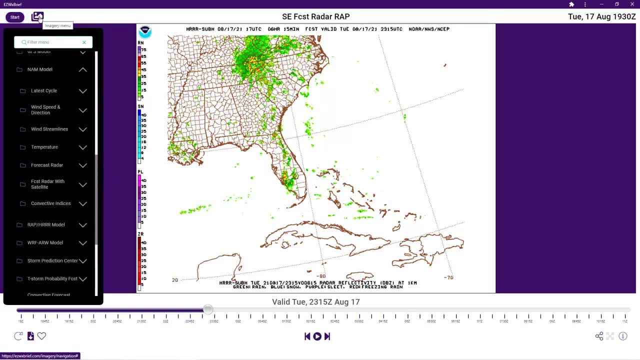 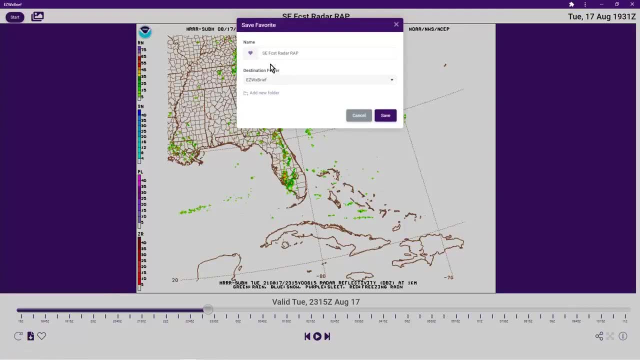 and if you find a specific model that you like and you find making use of it, go ahead and click on the heart at the bottom on the lower left. Then you can create whatever name you want. up here You can say it's the forecast radar.